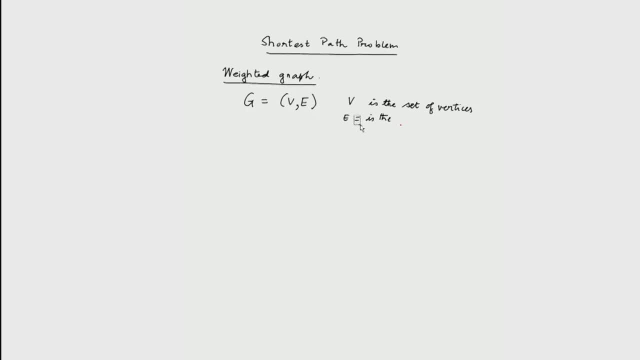 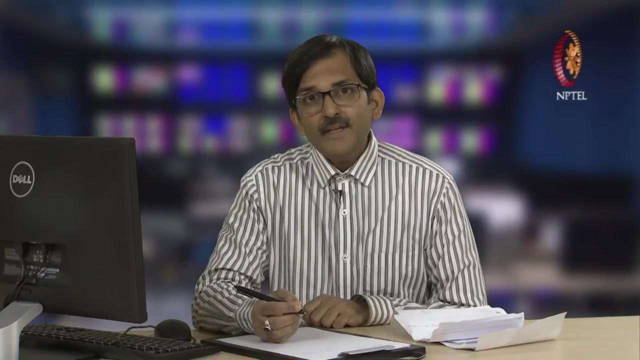 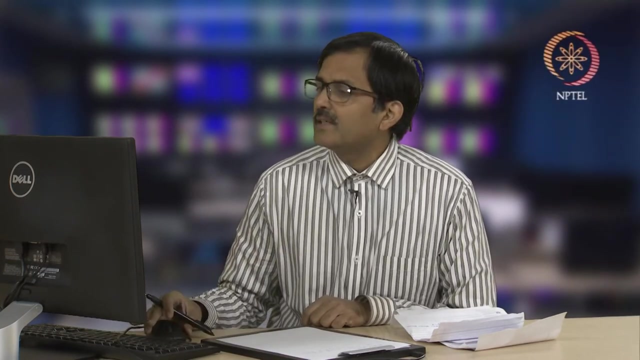 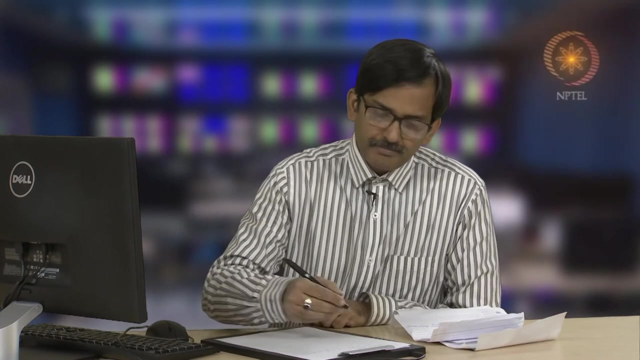 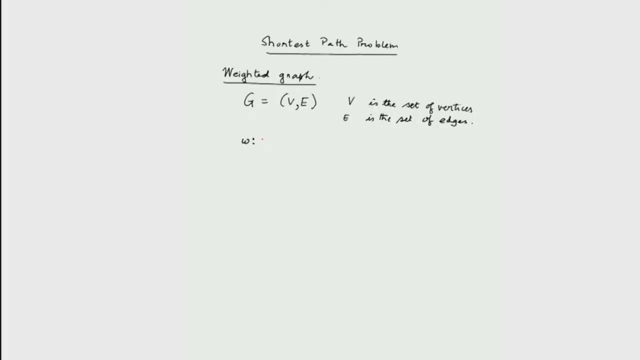 comma k, comma k, comma k g, g, Rudolph, g, g, g, g, g, g, g, d, z, g, e, 0, e, g, e, And in our discussion we will take the edge the weights to be greater than 0. So strictly speaking, we consider a function from e to positive real numbers. 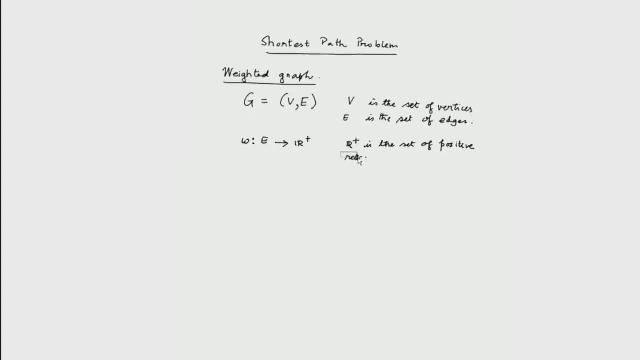 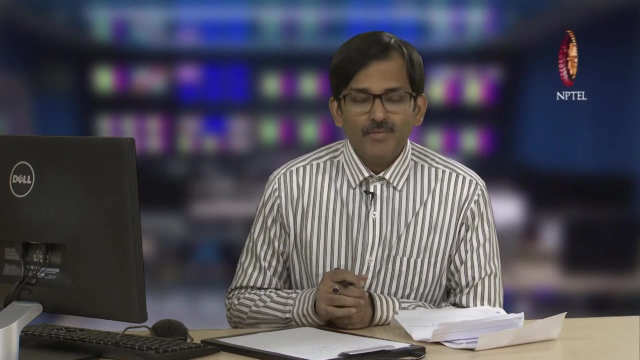 0.. So we consider functions from e, the set of edges, to r plus, where r plus is the set of positive real numbers And these. this function is called the weight function and individual values of this weight function will be called the weights function. 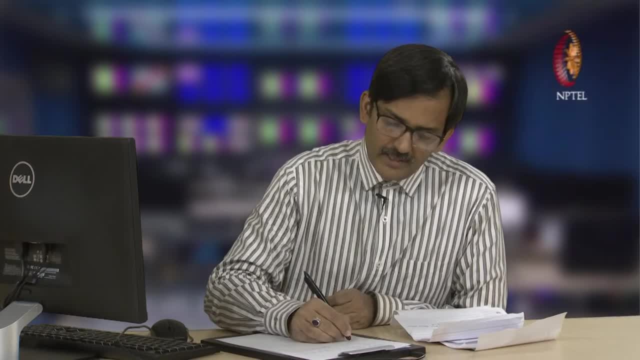 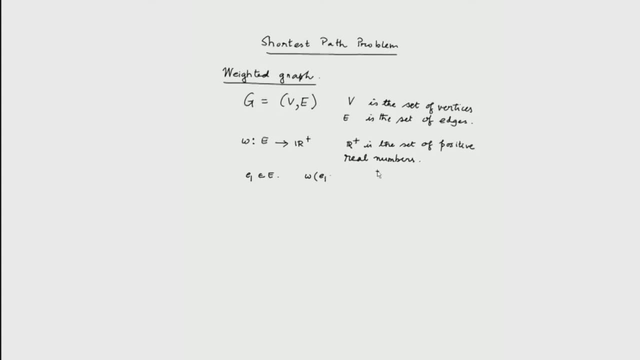 For example, suppose we have an edge e 1 belonging to e. we can operate the weight function on this edge e 1 and we will get w e 1, which is a positive real number and which will be called the weight of the edge e 1.. Let us look at an example. let us consider a graph. 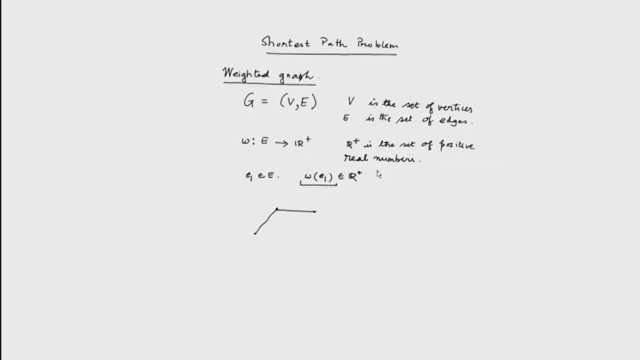 like this. Suppose these are the vertices a, b, c, d and e and the edges, suppose e 1, e 2, e 3, e 4, e 5 and e 6.. Now each edge are assigned to some weights. possibly the edge e 1 is assigned to 1,, 2,. 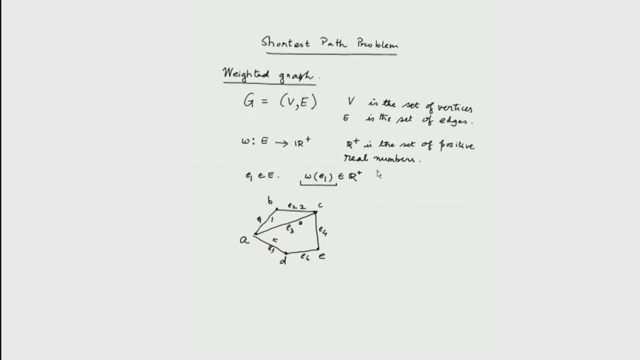 3,, 5,, 4 and 7.. So that means that w e 1 or, in this case, since this is a simple graph, we can also say that w a b. So, for example, w e 1 is equal to 5, w a b is equal to 1, w e 2 is equal to w b, c is: 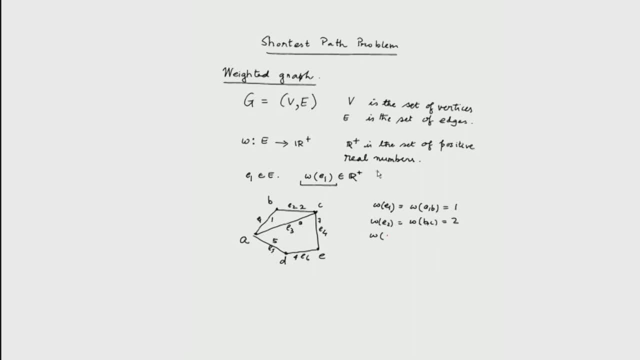 equal to 2, w a c, w e 3, w e 3 equal to w e 4 and w e 4, w 6.. Now each edge is a positive: 2, a c equal to 3, w e 4 equal to w c. e is equal to 7, w e 5 equal to w a d equal to. 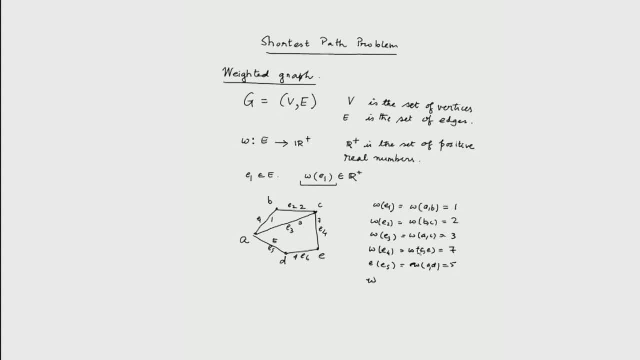 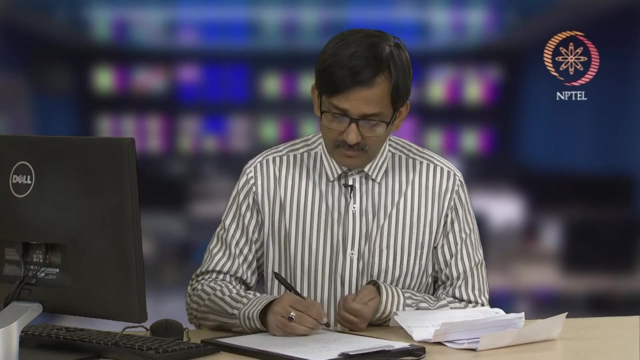 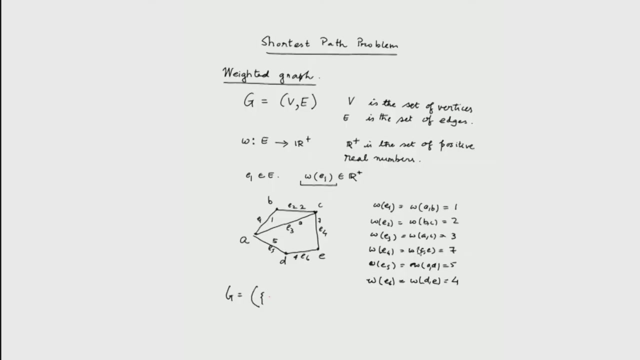 5, and w, e 6 equal to w, d, e equal to 4.. So these are the weights of the edges and this graph, which was originally g to a, b, c, d, e and edges e 1, e 2,, e 3,, e 4,, e 5, e 6.. These graphs, when we consider, 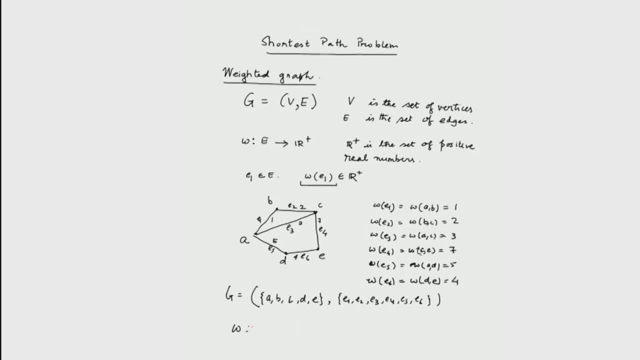 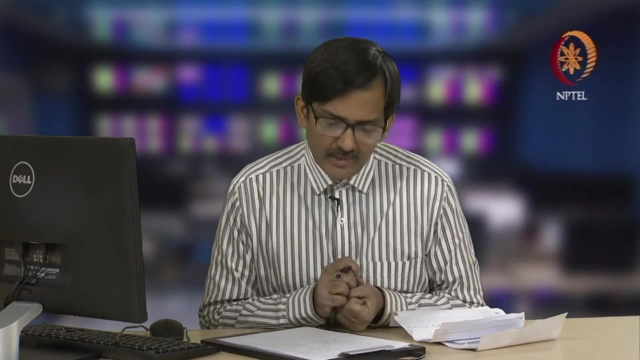 the function w from e 1 up to e 6, that is, the set of edges to the set of real numbers defined as over here, becomes a weighted graph. Now our problem here is that suppose I am given two vertices in a weighted graph, how do we find out the shortest path from the 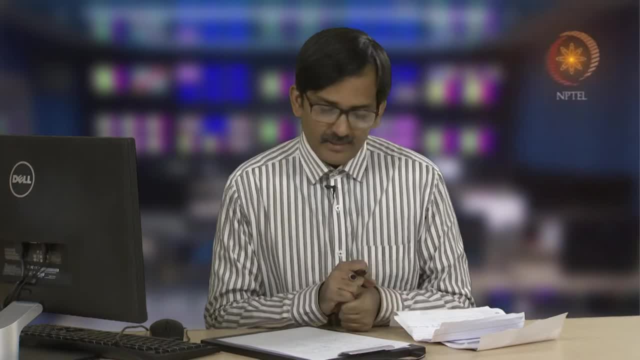 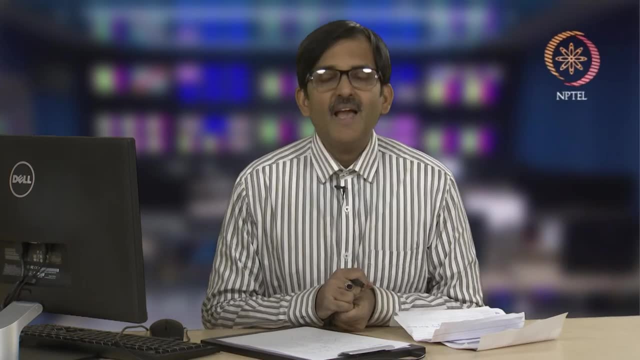 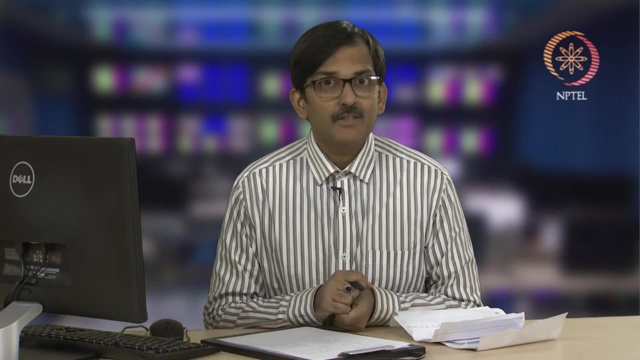 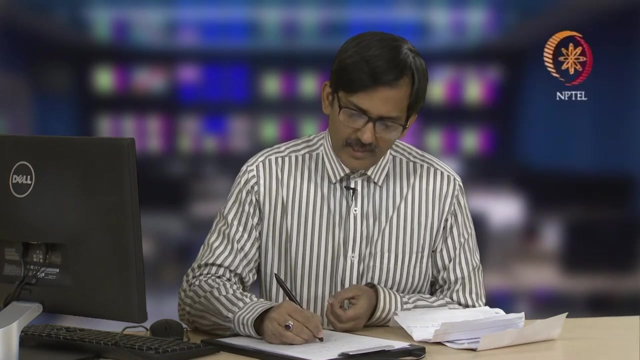 first vertex to the second vertex, and by the shortest path I mean that a path such that if we add up all the weights of the edges belonging to the path, we will get the smallest value. If we look at the graph that we just drew over here, if we consider the vertices a and 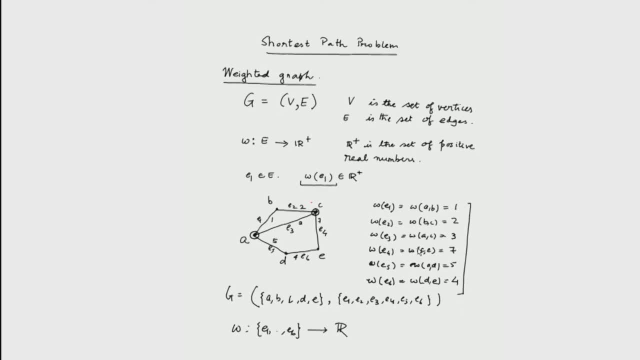 vertices c And suppose we want to go from vertex a to c. we have got at least three paths. one is a to b and b to c. we see the total. the total weight is 3.. So we have got a to b. 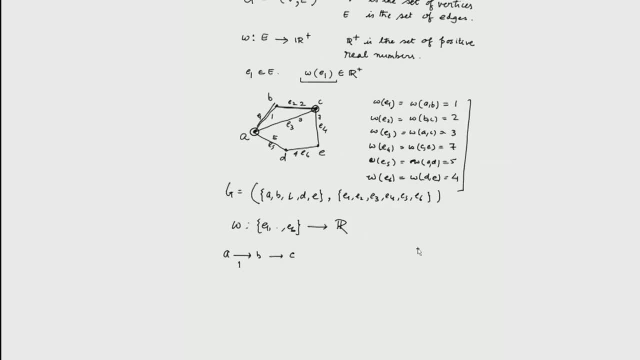 and b to c. a to b is 1, b to c is 2.. So the weight is 1 plus 2, which is equal to 3, the total weight- or otherwise we we could have gone from a to c- the total weight is: 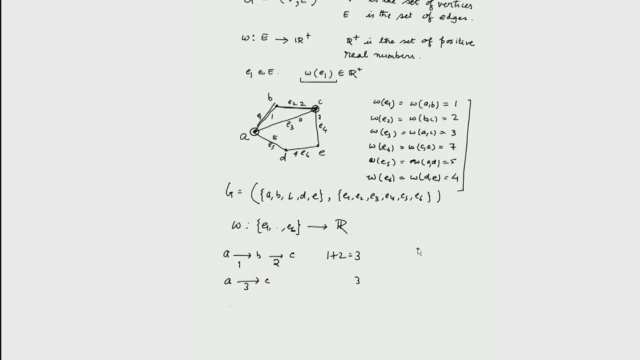 3.. Well, and the other possibility is: from a to d, d to e to b to c, that is, I will have 3.. All right, all right. so the total weight is 1 plus 2, which is equal to 3.. The total 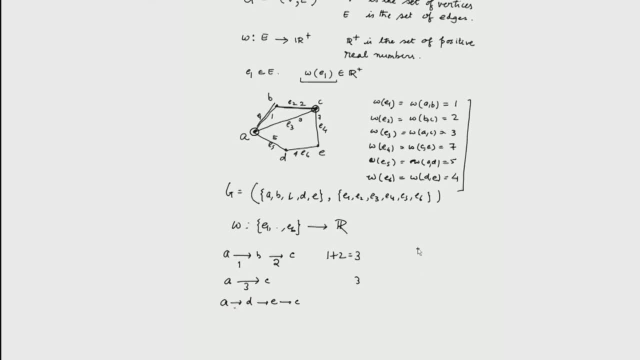 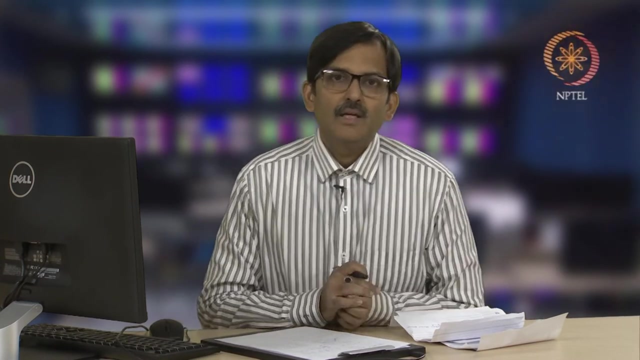 e, e to c, a to d is 5, d to e is 4 and e to c is 7.. So the total weight is 5 plus 4 plus 7, equal to 16.. Now, of course, the shortest paths are this or this, Now, this: 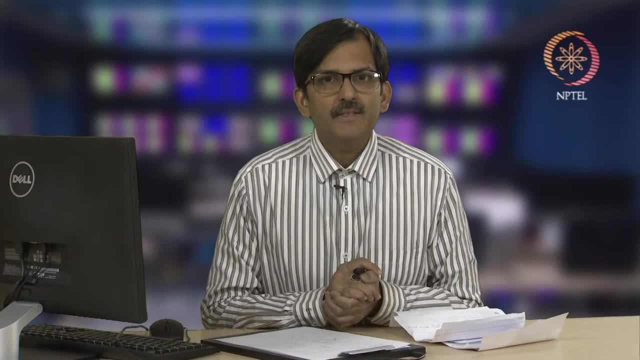 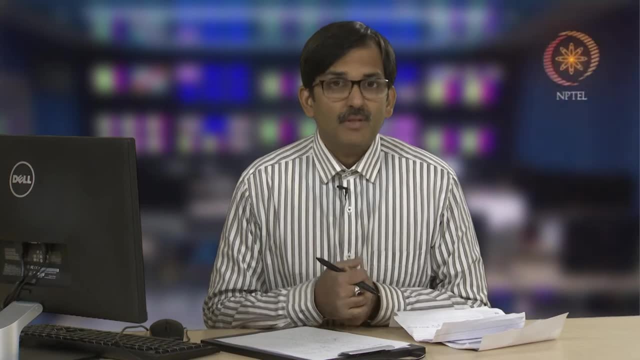 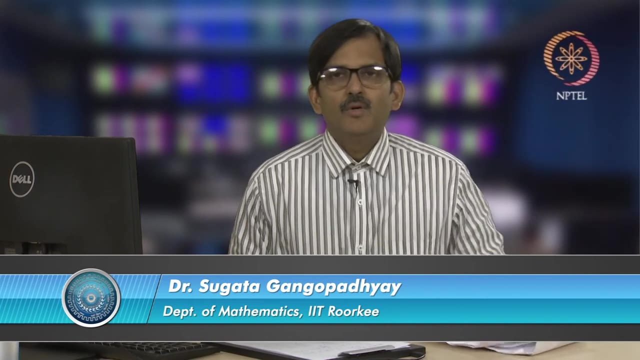 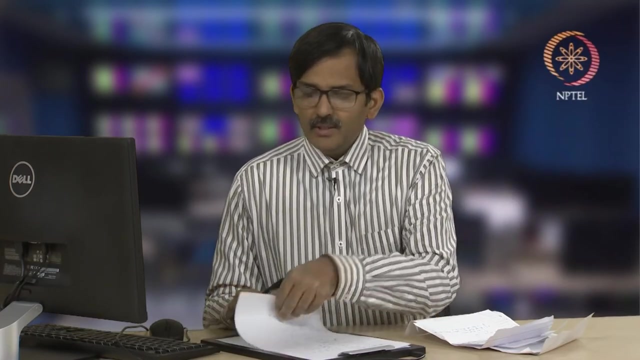 is a small example and the graph is quite simple. That is why, by observing the graph and checking the weights, it is possible to find out the shortest path, But it may not be so when the graph is complicated. we need an algorithm, and Dijkstra's algorithm precisely. 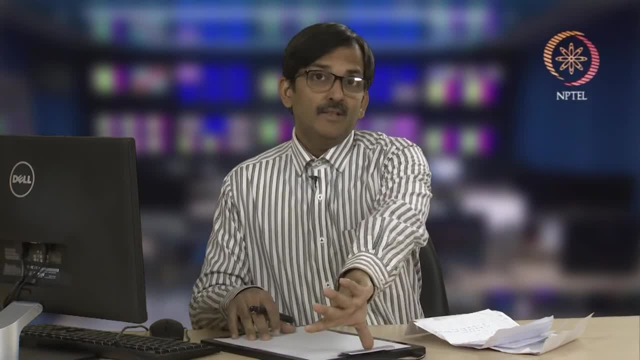 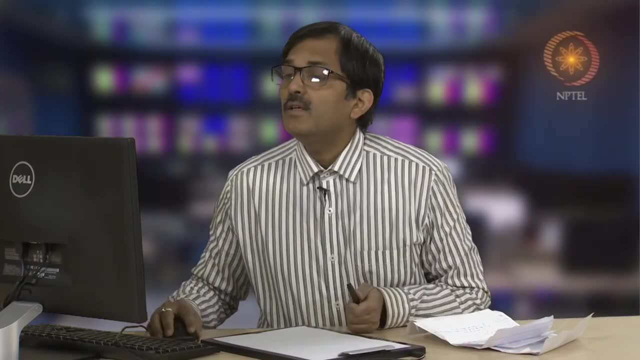 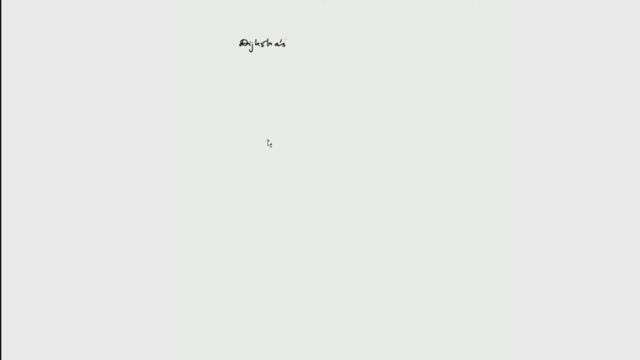 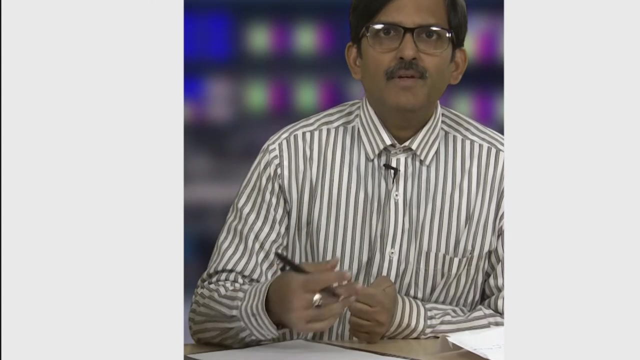 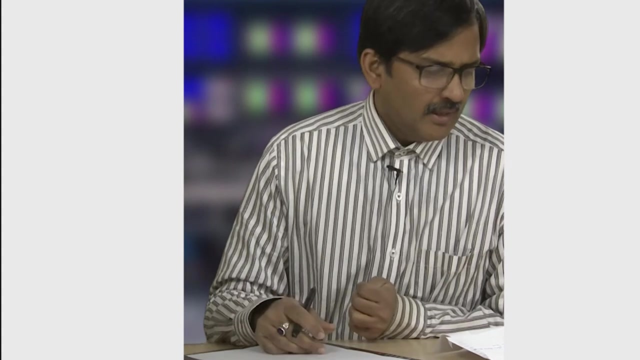 gives us That, so to say, Dijkstra's algorithm gives us shortest path between two points. Now we move on to Dijkstra's algorithm. Suppose V have got a graph where we are labelling the vertices by A, B, C, D, small letter and. the edges from one vertex to the other by a comma root a, the R T側. The having googles here be ONE V and 15 V. so once on A To match this point, G, G and 0 is E to d, is 1 to E plus. 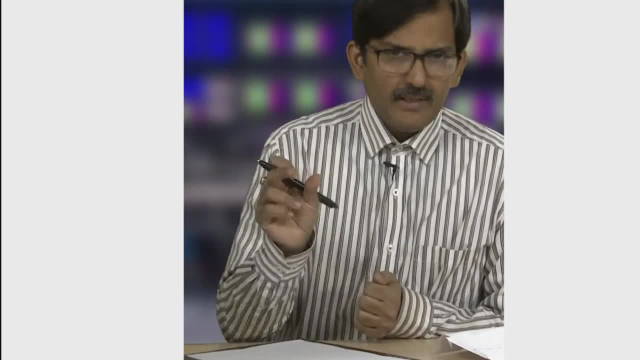 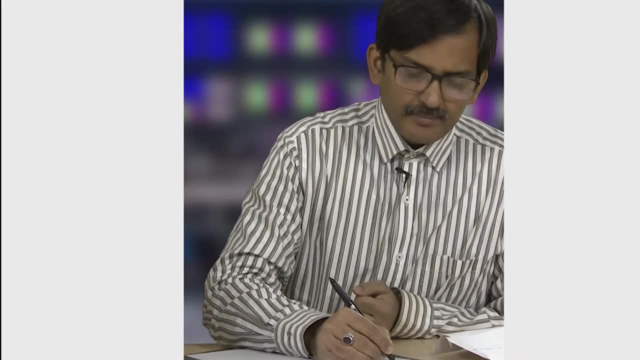 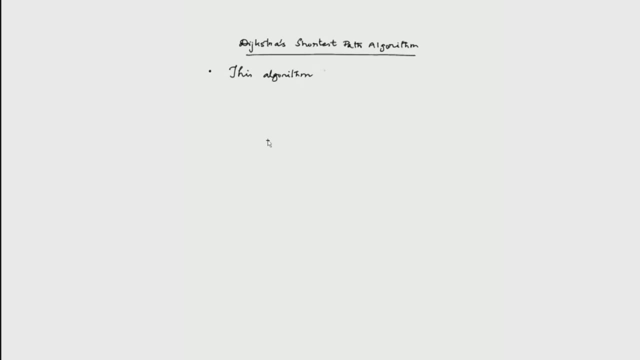 L is 0.. Jerome Levin, commentator, shed light and warning. or, as Now, what about you, Dijkstra? help by an ordered pair. So now this algorithm finds the length of a shortest path from the input vertices a and z. a and z. 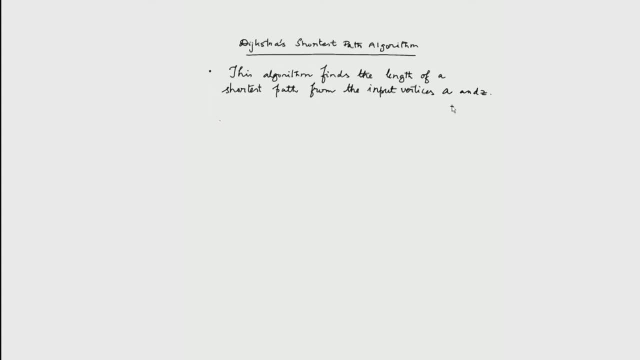 In a connected weighted graph. the weight of the edge i j is w i j, which is taken to be greater than 0.. And the level of the edge i j, which is taken to be greater than 0.. And the level of the vertex x is denoted by L x. Now here. 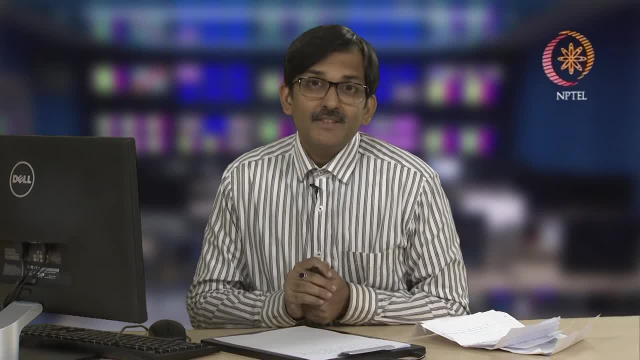 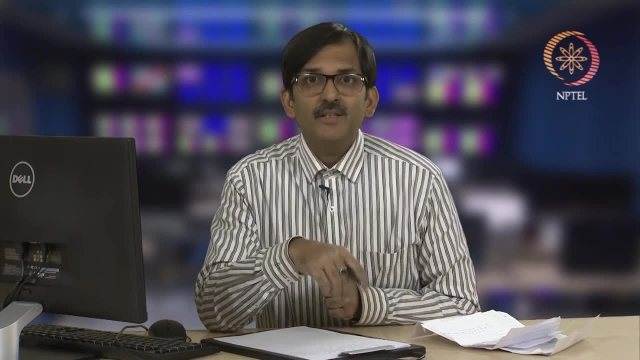 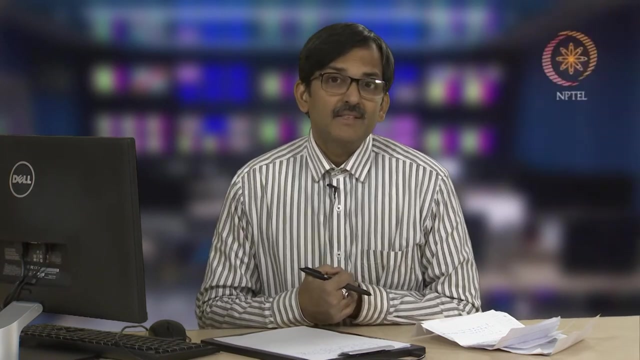 in this algorithm, to each vertex we assign a level which is greater than or equal to 0, which initially keeps on changing and after that comes to a fixed level, And that level gives us the shortest length path, by which I mean the path for which the sum of 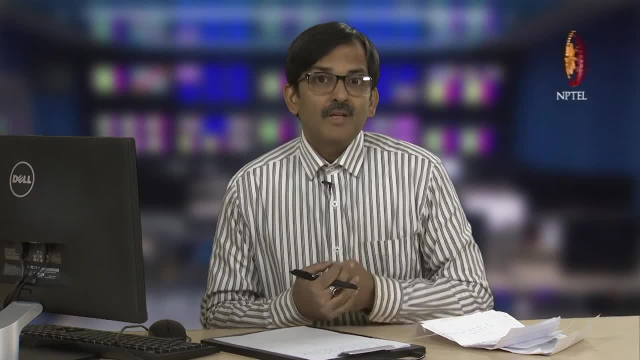 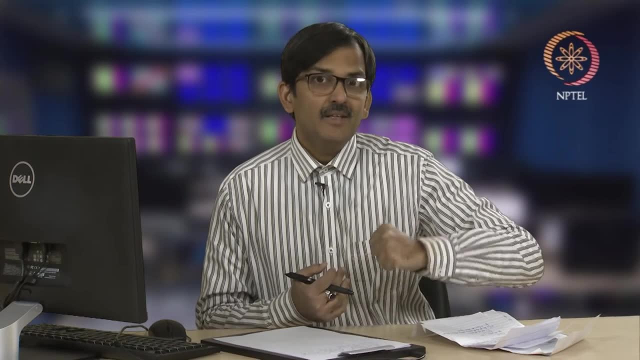 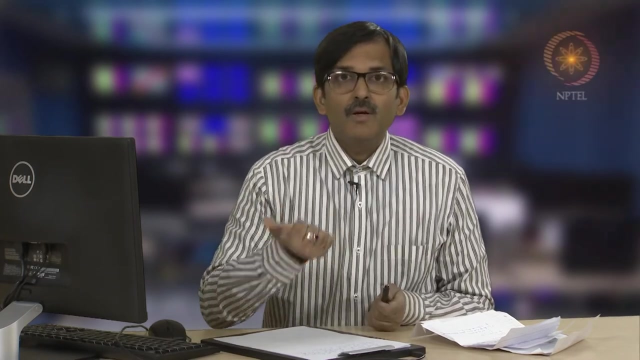 the weights is the smallest, The shortest length path from the point a. it is a vertex a to x And this length path is given by the line a, which is the shortest length path from. and this labels will keep on changing and ultimately, when we take the first input as 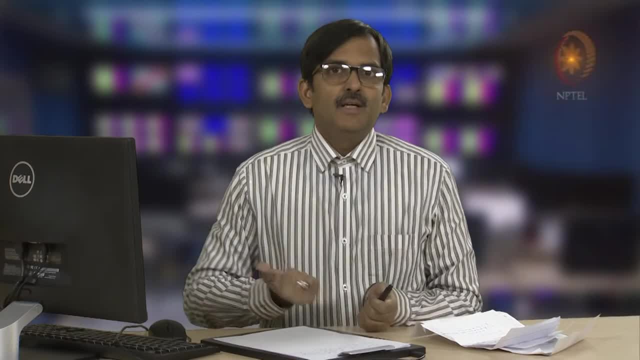 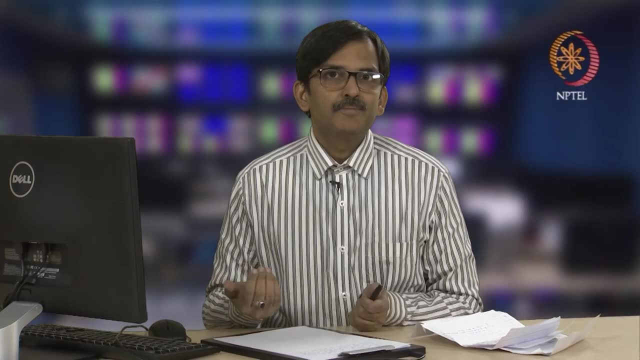 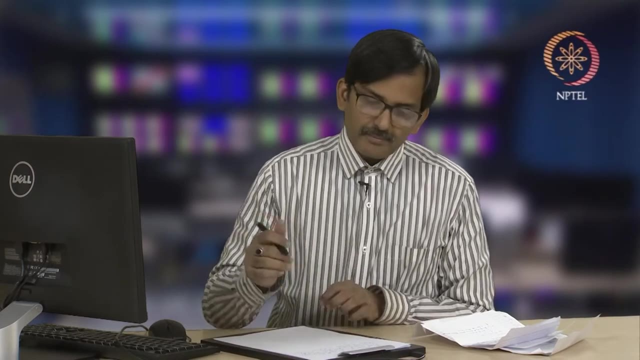 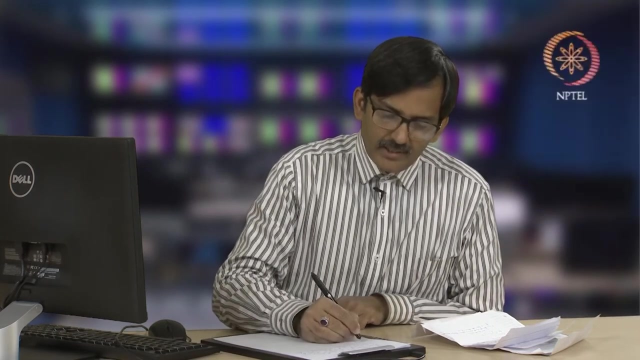 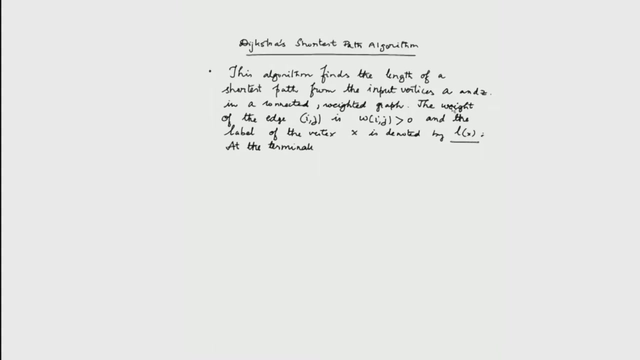 a, that is, we want the shortest path from the, from the vertex a, and when we start calculating the labels, at the end of the algorithm the label corresponding to z will give the length of the shortest path from a to z. So the labels are denoted by LLx at the termination. 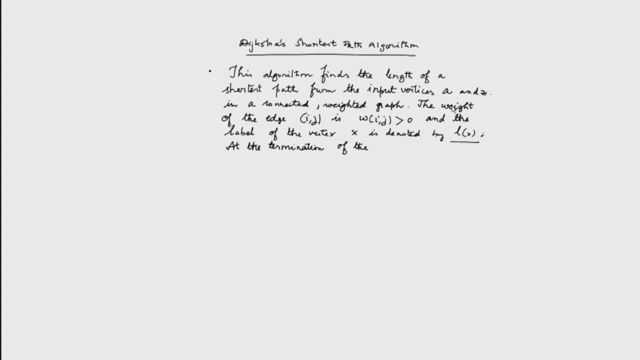 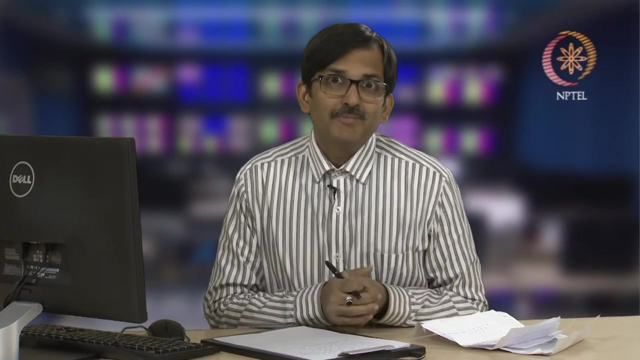 of the algorithm. Lz. Z is the length of the shortest path from a to z. Now let us start discussing the algorithm. So first step is input. Our input is a connected weighted graph in which all weights are positive and vertices a and z. So we have got two inputs, so to say. one is the graph on which we would. 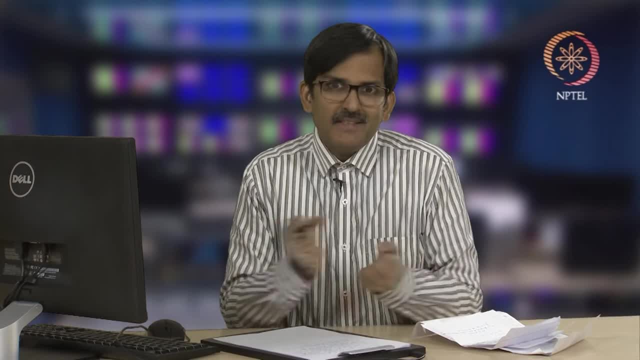 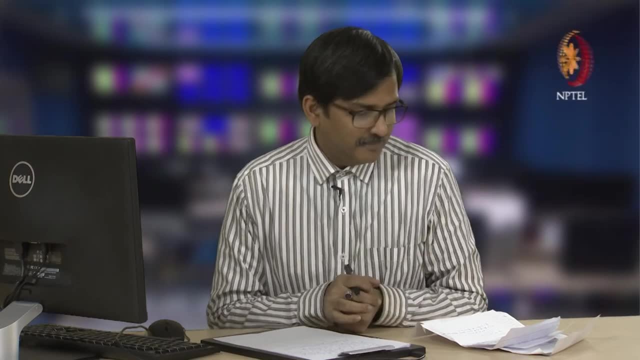 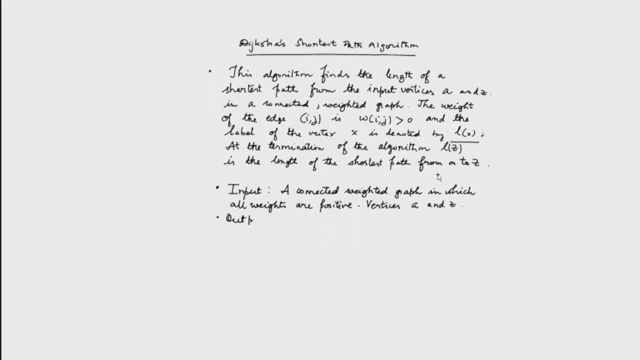 like to apply the algorithm and two vertices in that graph, between which we want to know the shortest path. Now the output is L z, which is the length of the shortest path from a to z. So this is the length. Now we come to the algorithm that we denote by Dijkstra W. This W is the weight function. 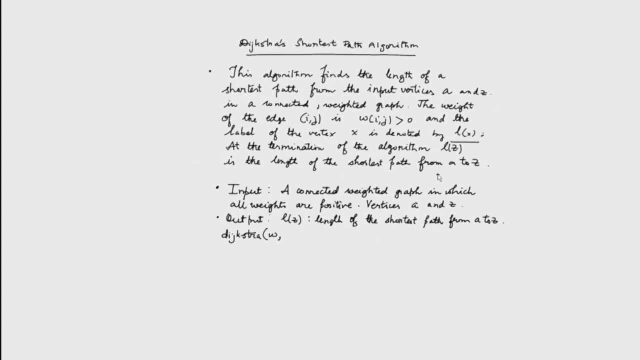 of the graph G that we are using, and a, z and the function L, which we will see how to compute Now. in first step, we will put L a equal to 0 and, for all vertices, x not equal to a. L x is infinity. . . . . . . . . . . . . . . . . . . . . . . . . . . . . . . . . . . . . . . . . . . . . . . . . . . . . . 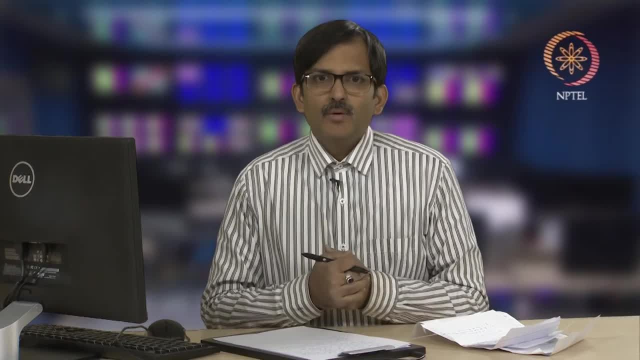 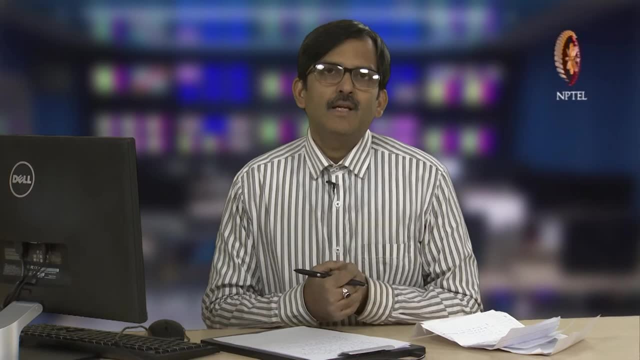 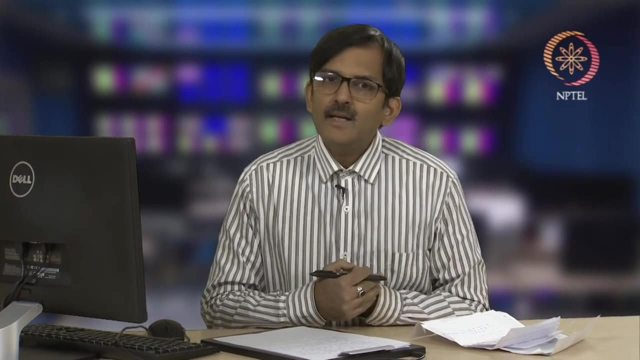 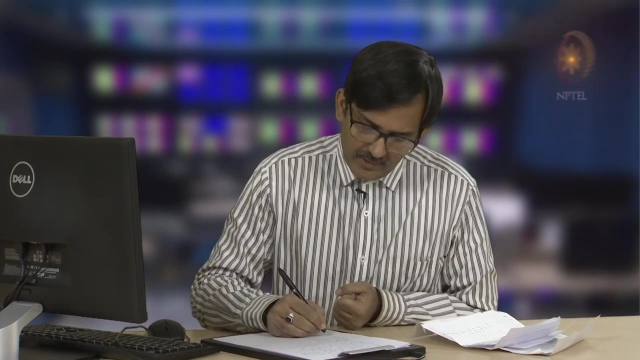 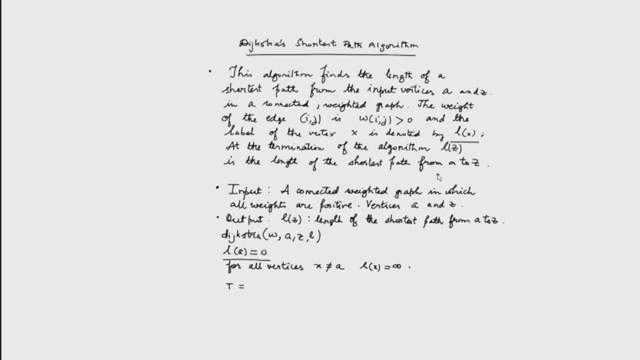 Thank you. Other than no, we leave it at set of vertices and then we will process this T. Now, in the first step, we come like this: that is, while Z belongs to T, we start this loop. choose V belonging to T with T. 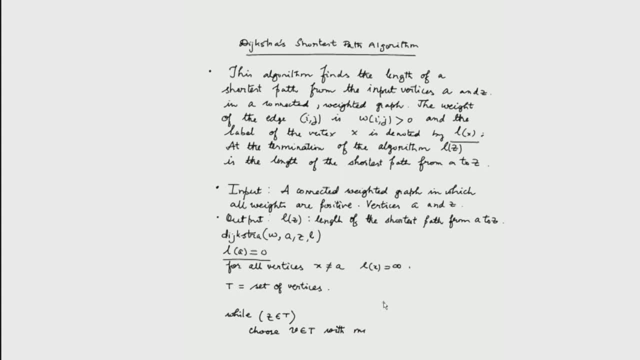 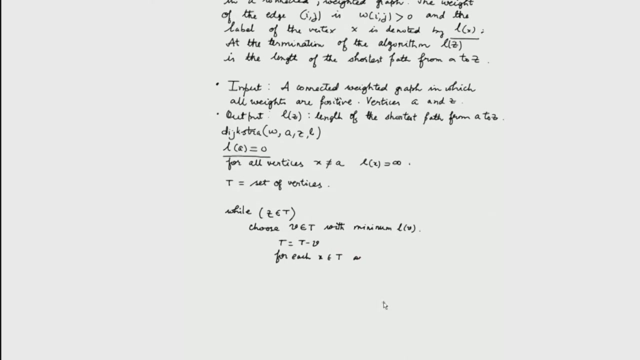 Minimum L V, and then remove V from T and build up a new T, and then, for each x belonging to T, Minimum L V, and then remove V from T and build up a new T, and then, for each x belonging to T, Minimum L V, and then remove V from T and build up a new T, and then, for each x belonging to: 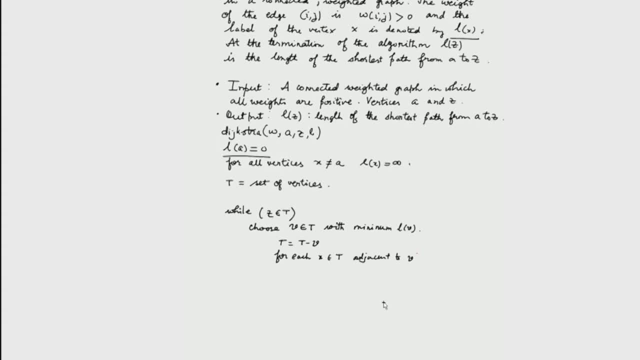 T and build up a new T, and then for each x belonging to T, and then for each x belonging to V, and then for each x belonging to T, and then for each x belonging to T appropriate size, L, V, and then properly assignment B to be. 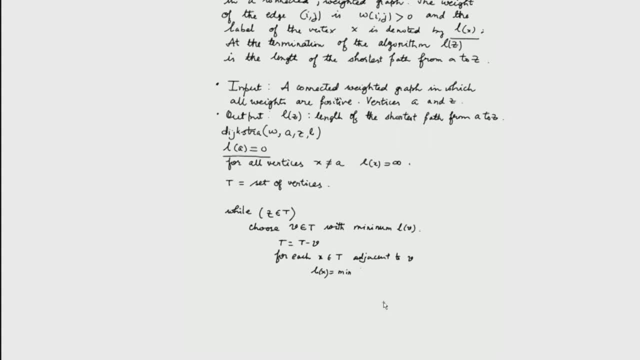 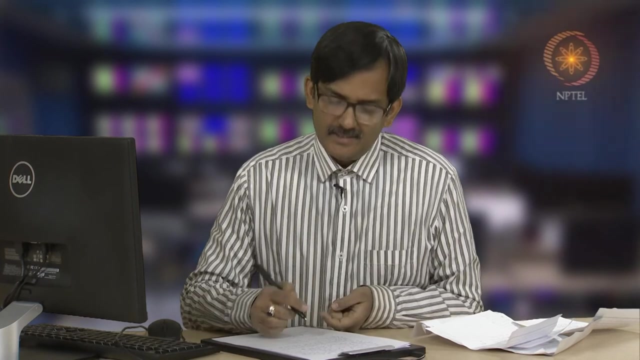 coloured in orange. The difference between the 하나�ue is that this kind of space, you know, is 2 by 2. now, how much space can be given? how much space should there be in this window? w, v, x and return. So let us see what happens. our starting set of vertices is a set of all. 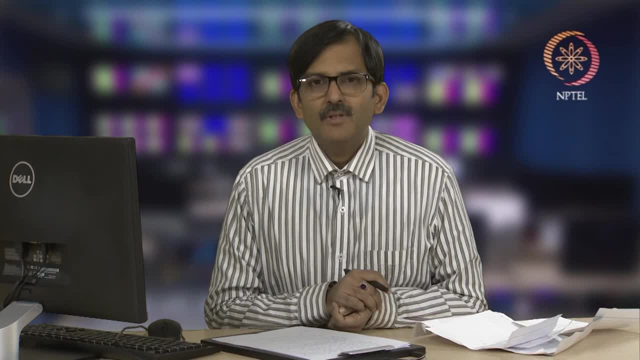 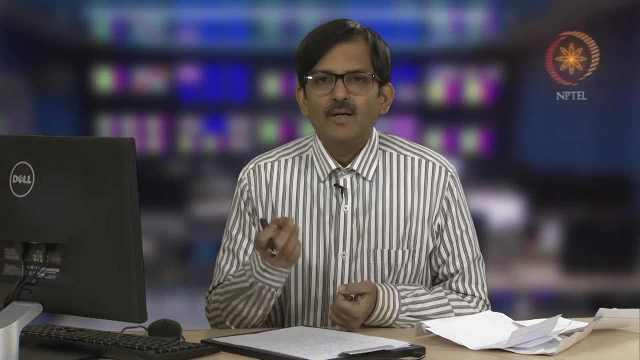 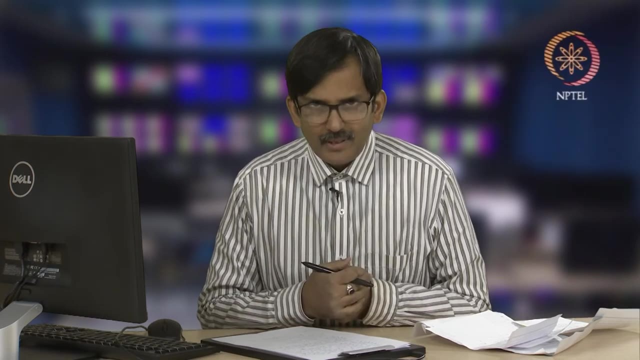 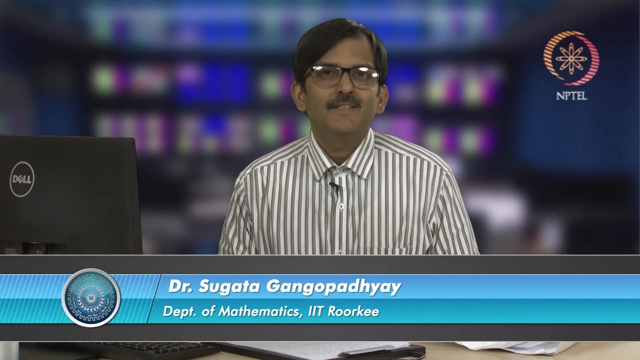 vertices and then among them, among that in T, we find the smallest weight vertex, that is, a vertex with the smallest level, and we choose it and then we delete it from T. So then we will get a set of vertices other than that vertex that we have deleted, and then 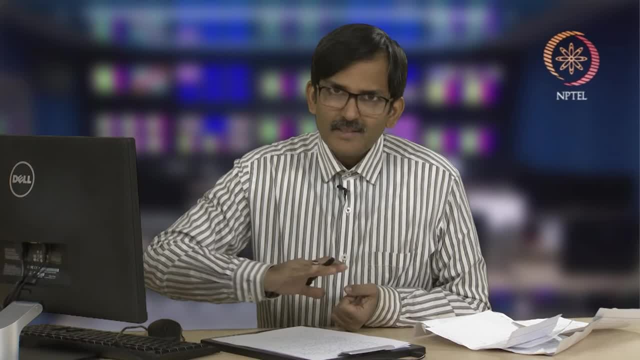 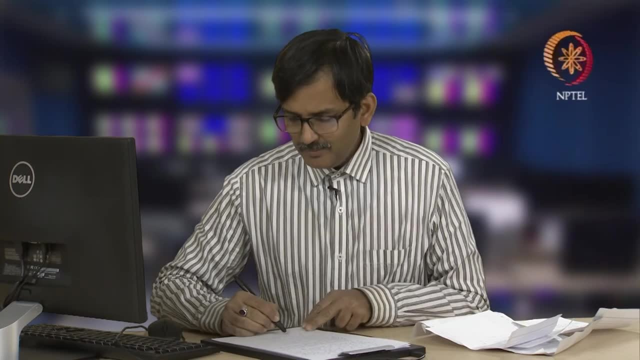 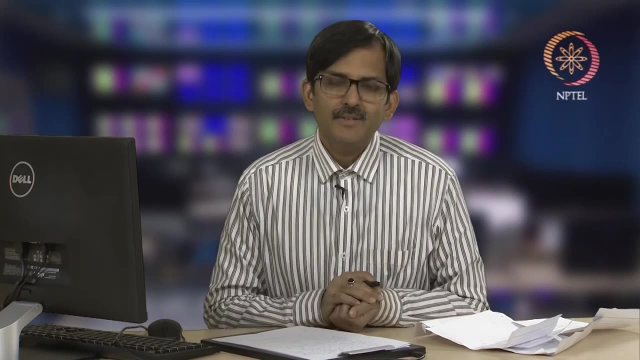 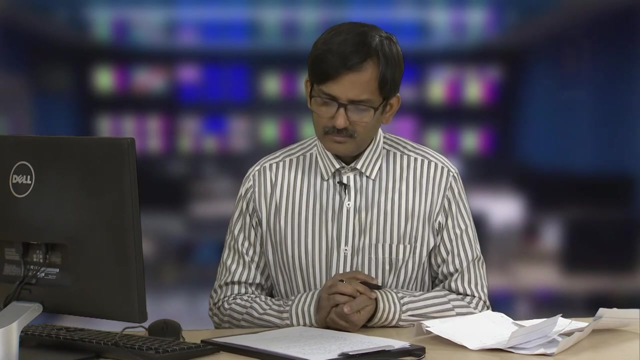 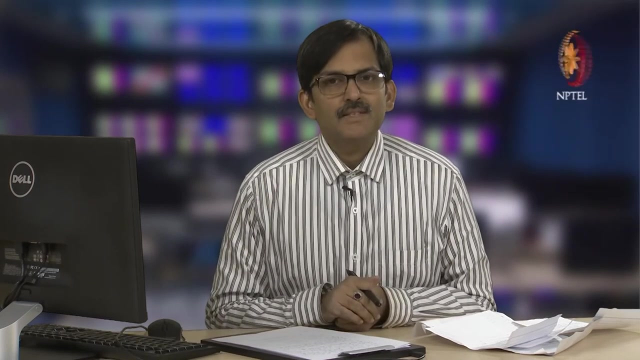 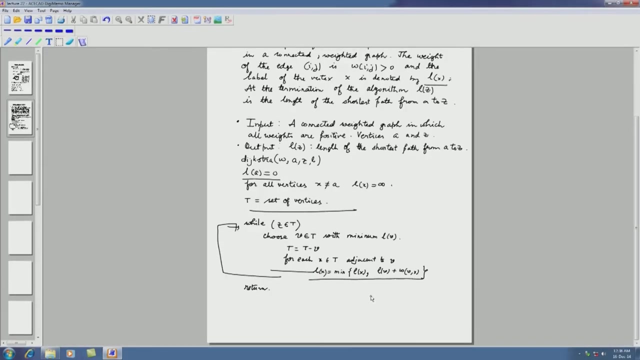 what we do is that we start scanning all the vertices which are adjacent to the deleted vertex and then we will calculate this quantity. So, after calculating this quantity, now my T is changed, I go again into this and we again do the same process. So this loop will keep on happening and this loop also will keep. 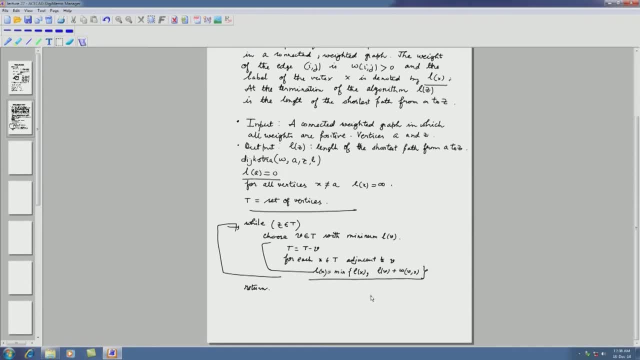 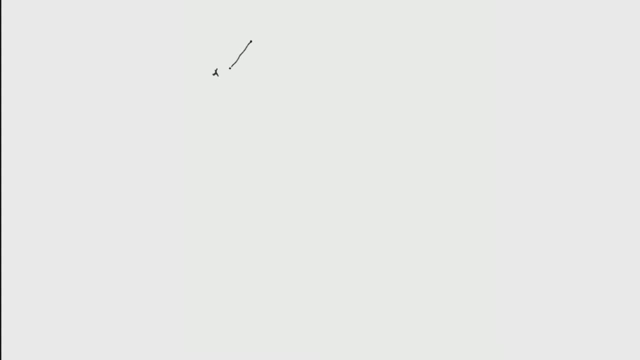 on happening. Please hold on for a moment Now. let us take an example to clarify this matter. This is a. A is connected to B and the weight is 3.. B is connected to D: the weight is 2.. D is connected to g: the weight is 3.. 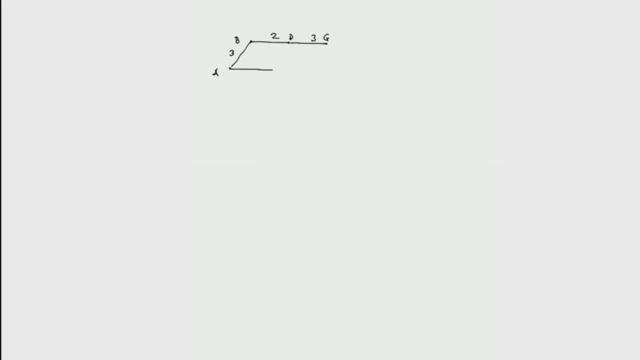 Then it is like this: So what is going to happen for the operation? t, A is connected, B is connected to E, the weight is 4, and here A, E, the weight is 9.. Now, here A is connected to C and the weight of the edge is 2, C is connected to E, the weight of the edge is 6.. 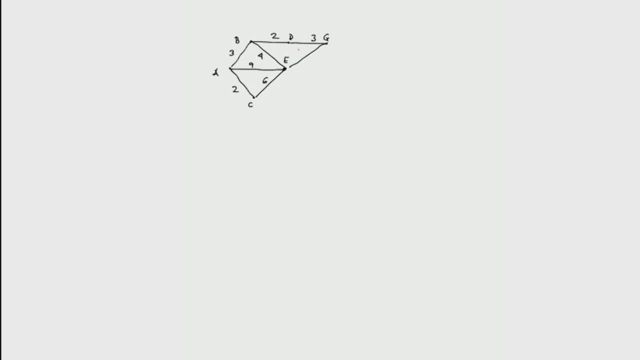 After that, E is connected to G, the weight of the edge is 1.. Now E is connected to H, the weight being 2, and C is connected to F, the weight being 9.. F is connected to H and G is connected to F, the weight being 1, and here G is connected to J, the weight being 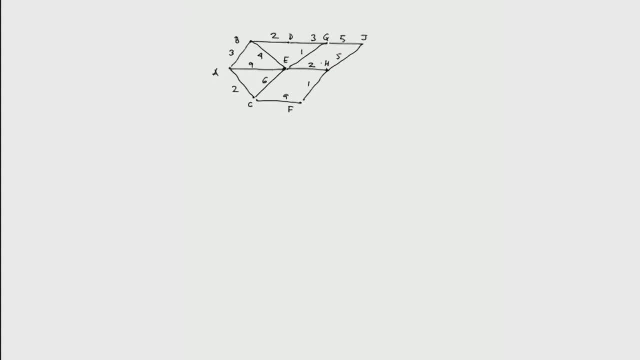 5 and G, J, the weight being 5. again, and here J is connected to L, the weight is 5, H is connected to L, the weight is 9, F is connected to I, the weight is 2, and G is connected to L, the weight is 9.. 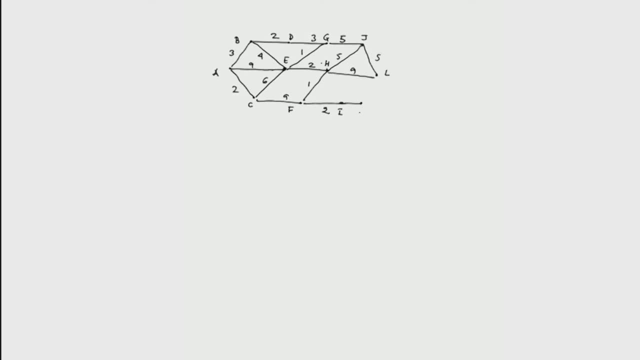 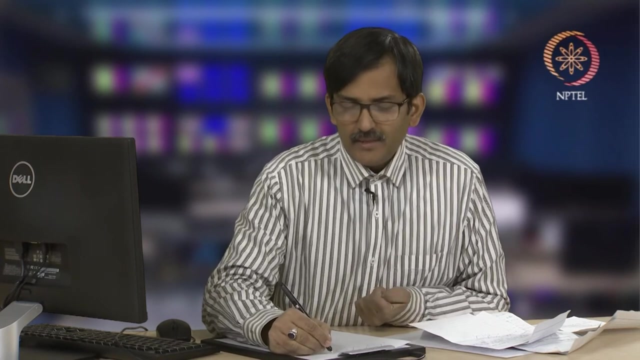 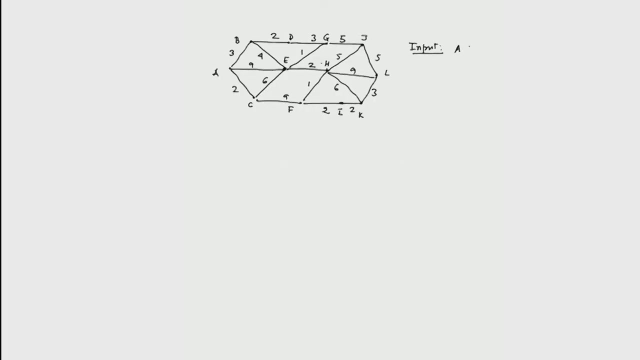 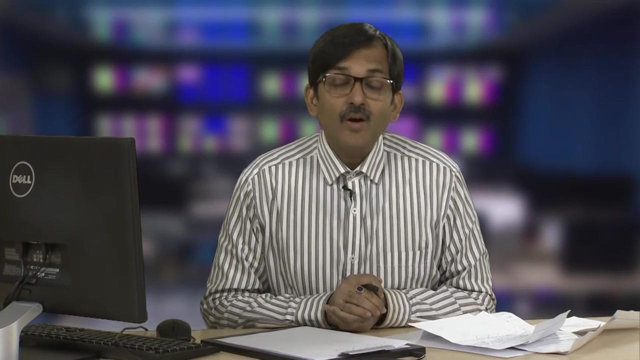 i is connected to k, the weight is 2. again h is connected to k, which is 6, and k is connected to l, which is 3.. Now suppose somebody tells me that my input vertices are a and l and I have to find out the shortest path between a and l. how do I start Now? let us go according. 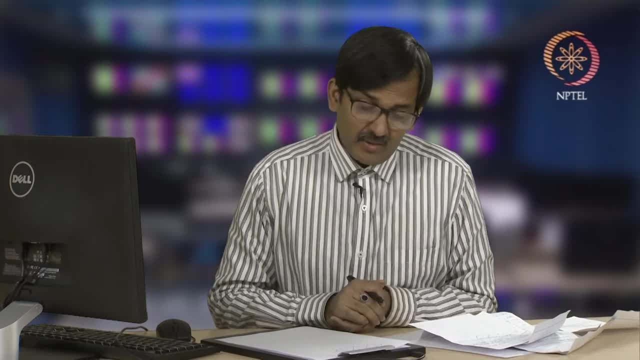 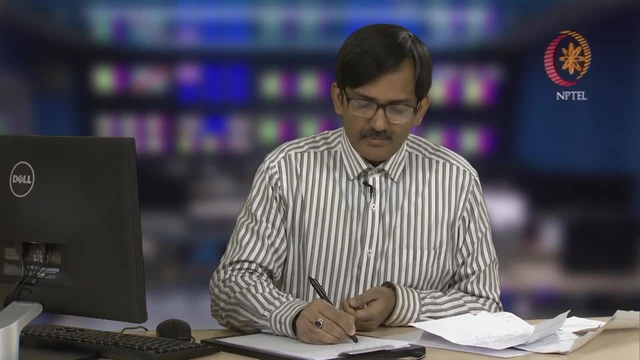 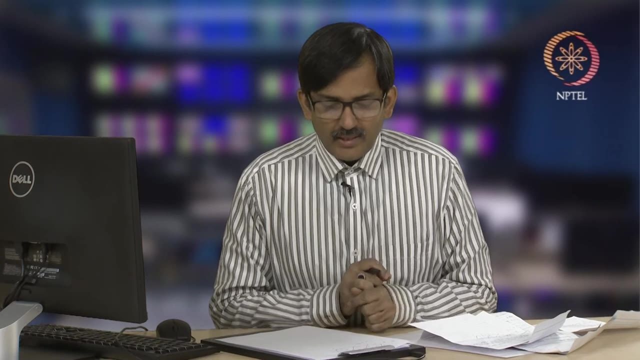 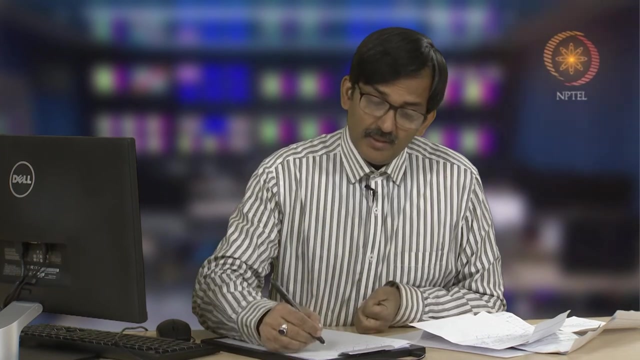 to the algorithm proposed by Dijkstra, step wise. In the first step, my t is a whole set of vertices of the graph given graph. So let us denote the graph by g Now, and then what I do before, that is that we, our starting vertex is L a, so L a is put to 0,. 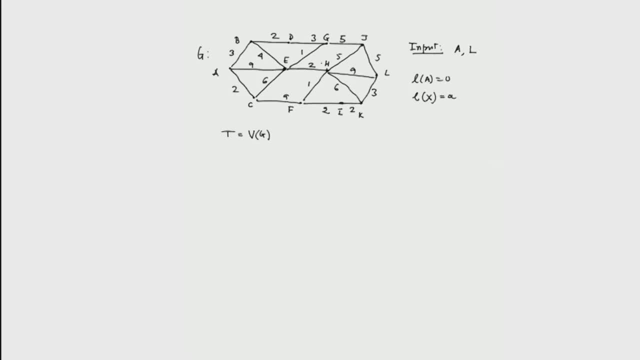 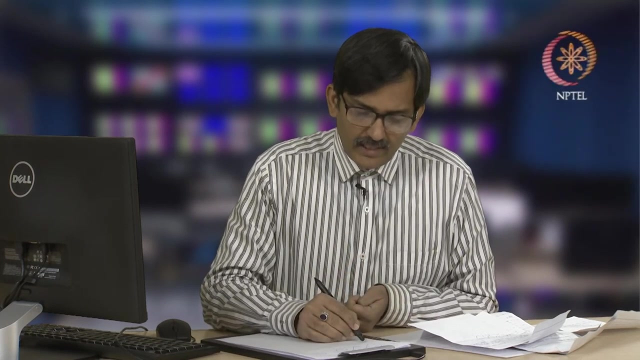 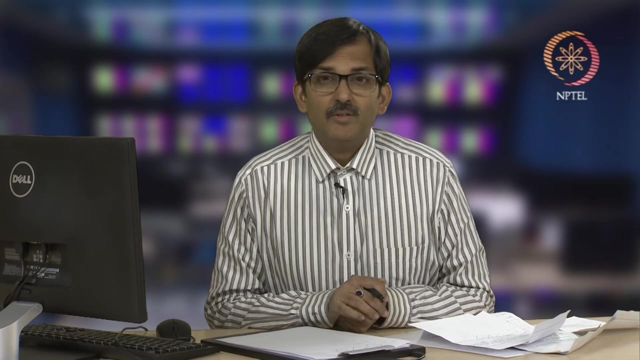 L of anything else, x is infinity for all x belonging to v, g minus L, So, other than a, all vertices are put to infinity. now we start with t. now, in the first step, we will consider the vertex which has got the least label value, and in this case it. 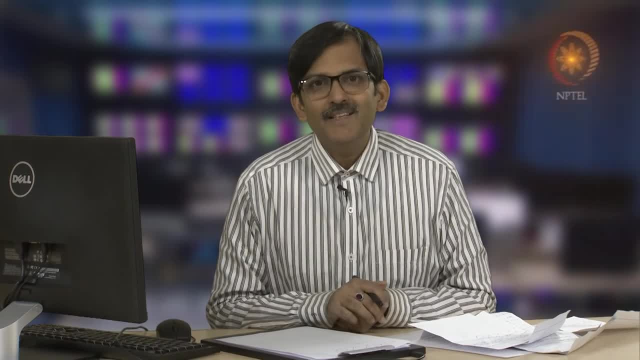 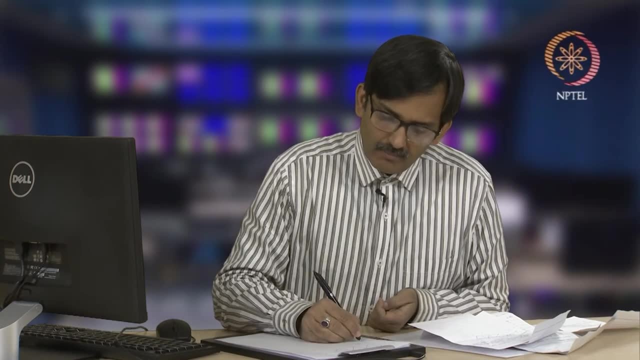 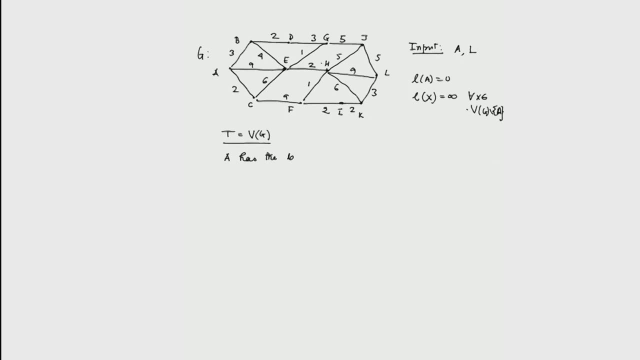 is a. so we will remove from t the vertex a. So see, this is the vertex a. this is the vertex. a has the least L value. so remove a from t. So I calculate t which is t minus a. So this is the vertex a. this is the vertex b. this is the vertex c. this is the vertex. 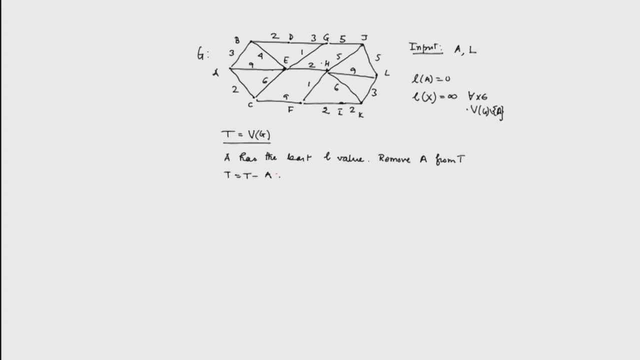 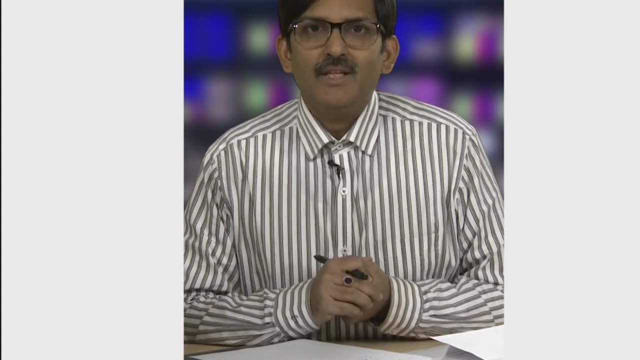 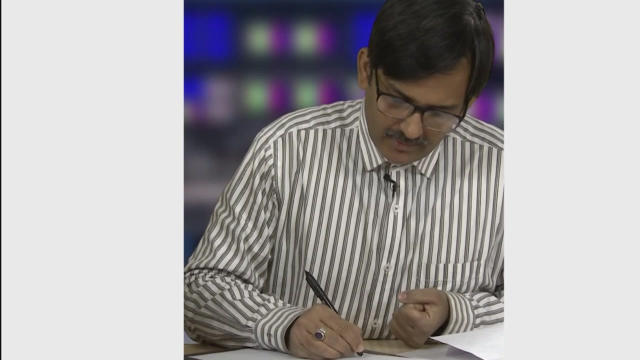 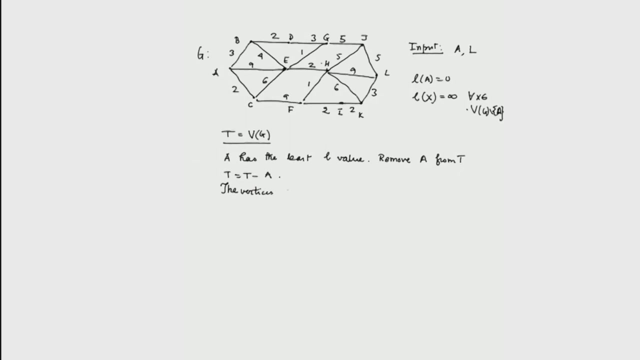 b Now, in that we have to consider all the vertices which are adjacent to a, the vertices adjacent to a. So this is the vertex a, this is the vertex b, this is the vertex c, this is the vertex c and that is the vertex b. Next, I will give you the whole architecture of this whole. 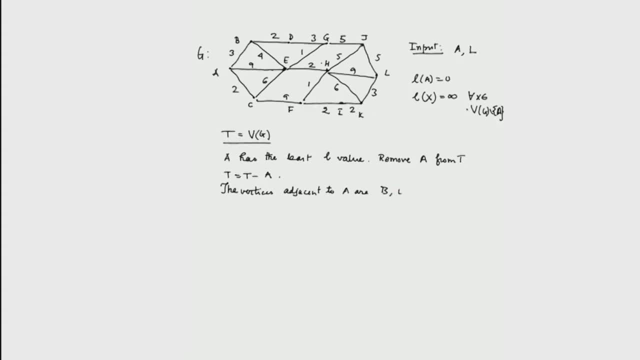 architecture: First set the vertex x, then the vertex y, another vertex y and set the vertex a. We use the form of x and we will convert the final Eigen value of this vertex to mé chuckle, that is Z, 4 plus about half, That is, minus a, minus L. that is, instead of through the vector. 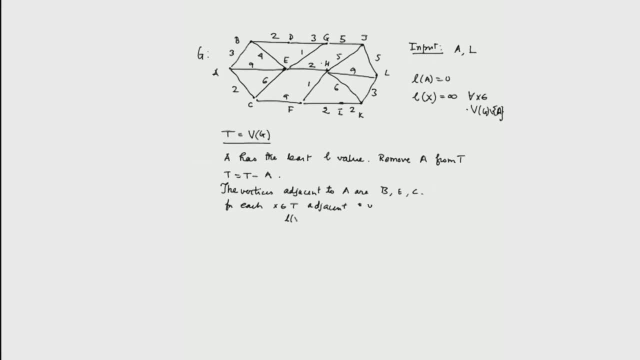 to v, L x equal to minimum L x, L v plus w, v comma x. So this portion of the algorithm is to be used now. So what do I do Here? my v is equal to a and v is equal to a, So 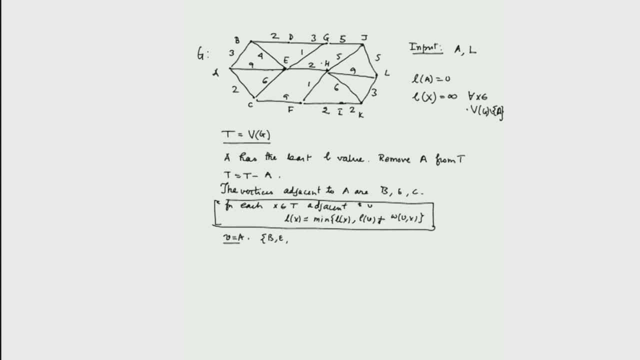 the adjacent vertices are b, e and c. So I calculate L of b to be minimum of L of b comma L of v, that is L of a plus w, a to b. Now we see that L of b is infinity and L 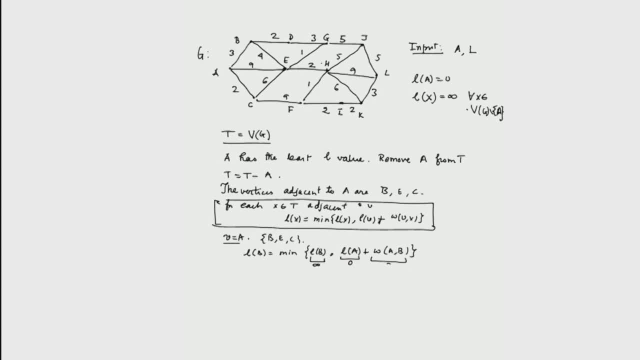 of a is 0.. W a b is 3.. So we have got a choice between infinity and 3.. So the minimum is going to be 3.. Then L of e is going to be minimum of L of e, and then L of a plus w a e, and using 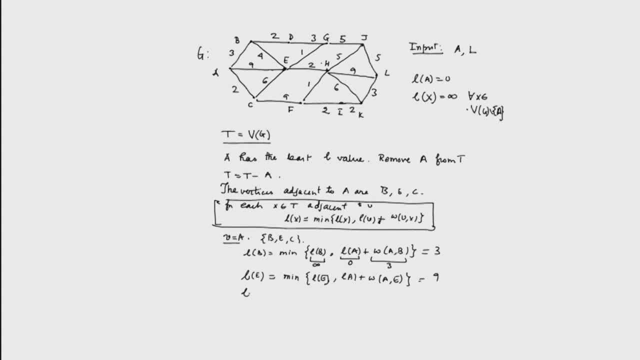 the same argument. it is going to be 9 and similarly, L of c is going to be minimum of 2, which is minimum of L of c, L of a plus w a c. Now we see that now we have a graph where I do not consider a anymore. So that is my. 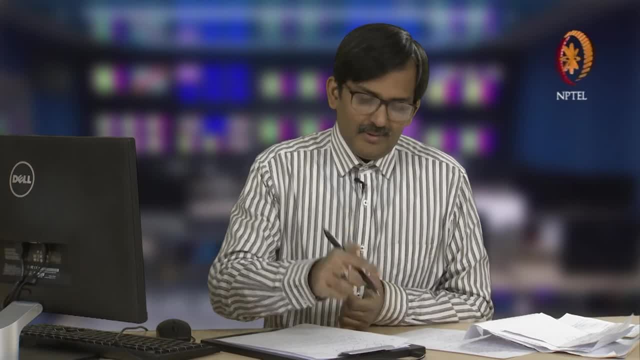 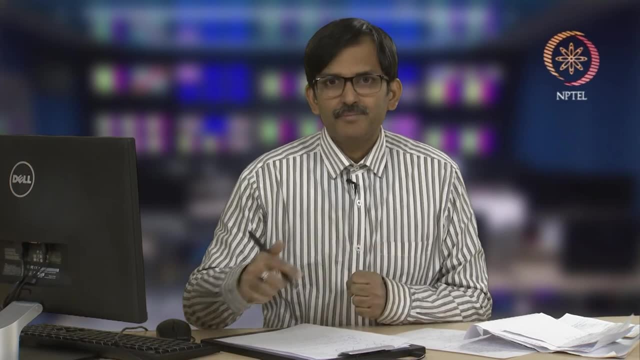 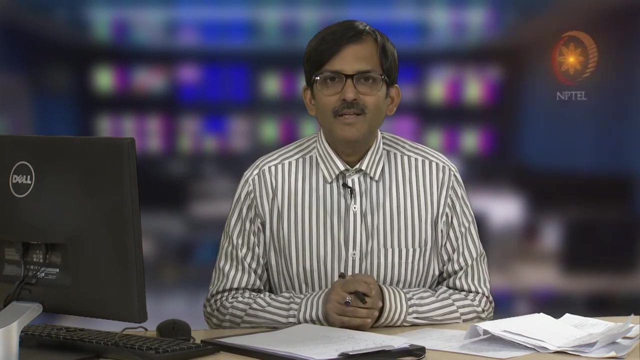 new t. So now I am going to Look at a star. So L of a plus w a x was 1, so that S of a plus w a x was 2.. So B of c is finished. So L of b is 1.. Now B of c is considered to be. 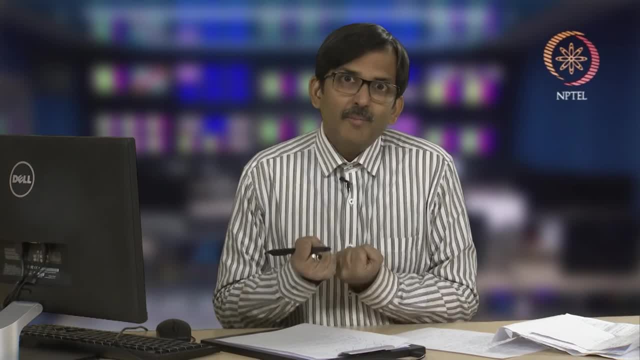 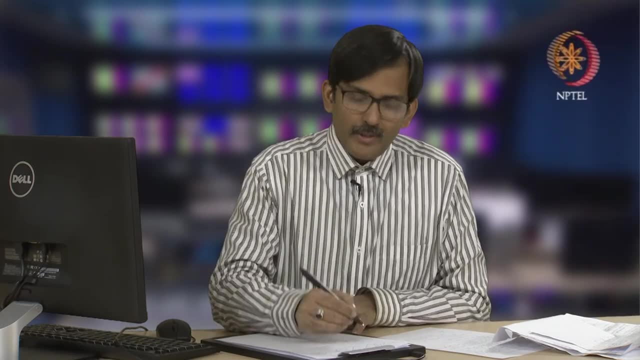 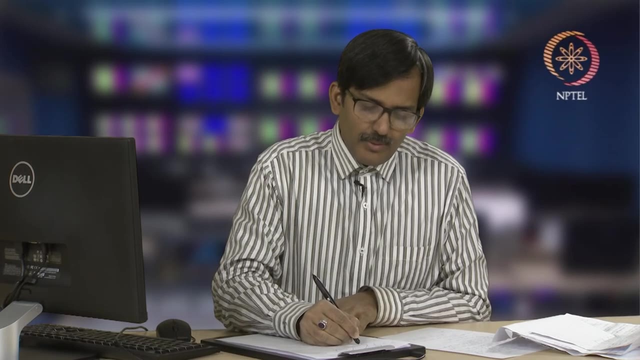 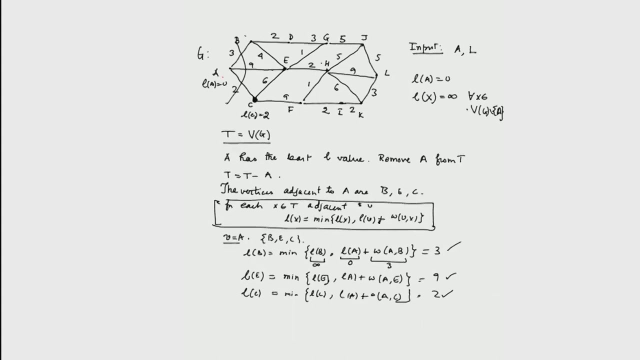 a negative sign. so that is 1.. Now let us see another value, which would be yesterday OK level, and that level value is going to be c over here, So I can put the level of c to be equal to 2. incidentally, level of a is 0 and then I will cut out c from t. So now 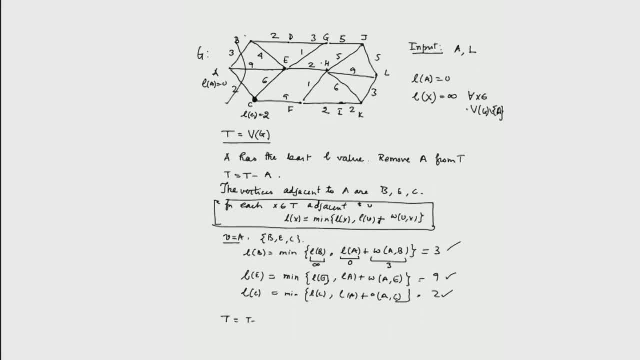 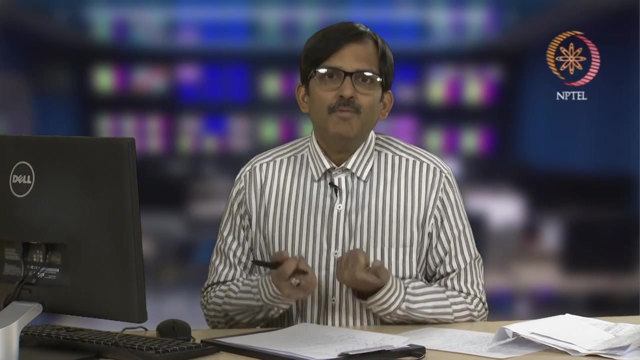 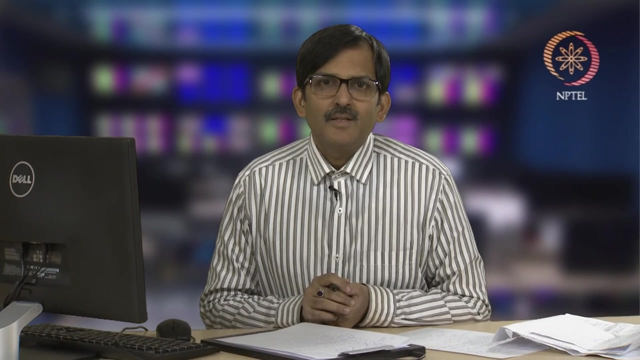 my t was t minus a, original t minus a. this is my t and now my. in next iteration my t will be essentially t minus a minus c. So I will have- I will also delete c Now. when I have deleted c now, I will calculate the new label values for the vertices adjacent. 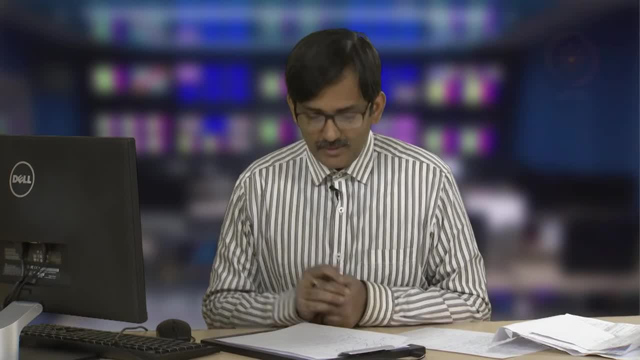 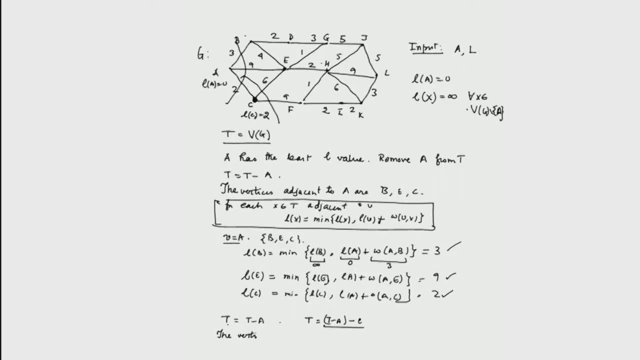 to c. Now, what are the vertices adjacent to c? The vertices adjacent to c are e and f. Now again, we will come to this step. For each of these vertices, we have to calculate this quantity. So l is the new label value. 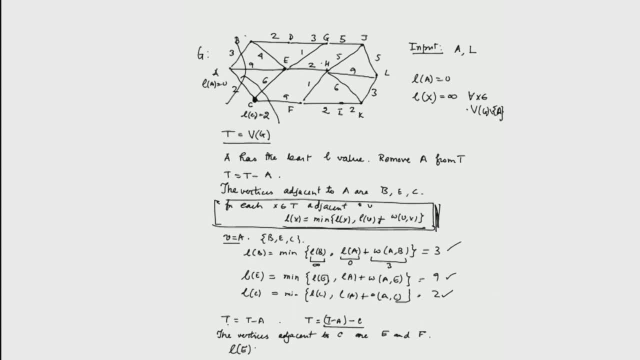 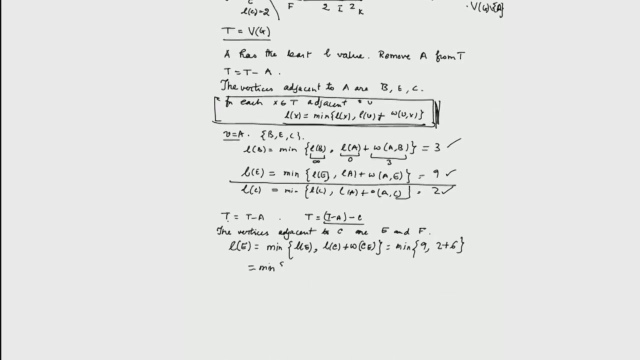 Now we know that e has a label value that is equal to 9.. So I have to take the minimum of l e and l c plus w c to e. Now that is minimum of 9.. And l c is 2 plus c to e is just 6.. So I have to choose between 9 and 8 and which is. 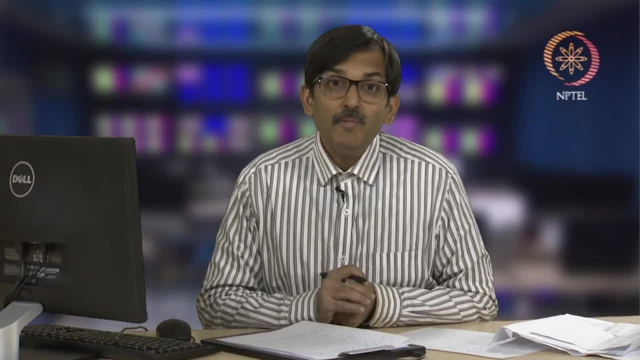 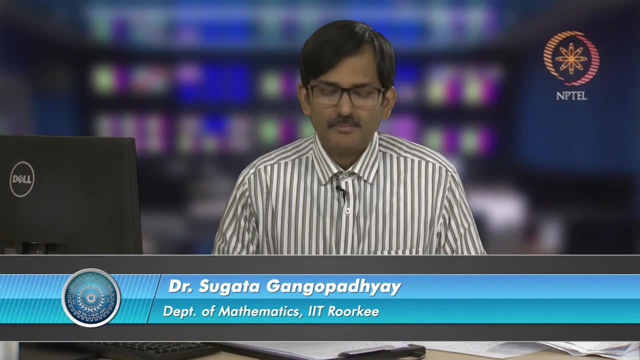 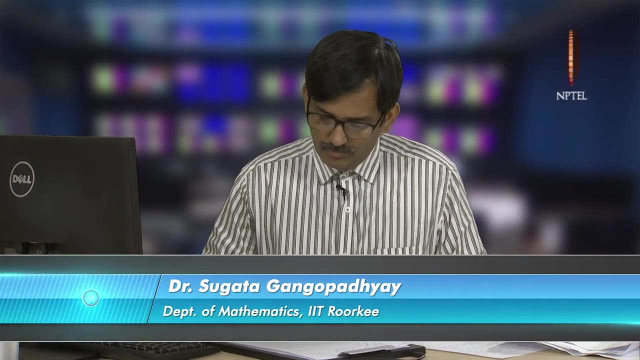 of course 8.. So we see that the label value of e has decreased, So we will put l c to. So we will put L e equal to 8 and L f equal to minimum. L f which is infinity, and L c plus. 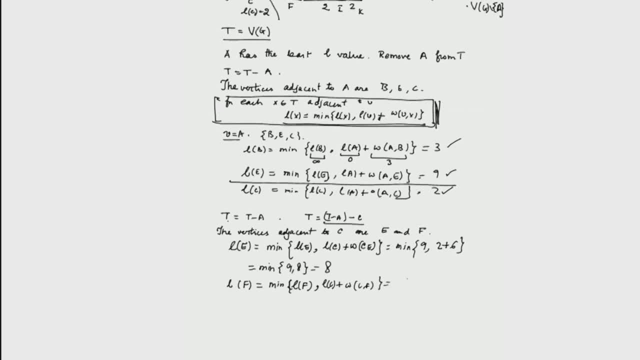 W c f. If we do L c plus W c f, then we have minimum between infinity, and L c plus W c f is going to be 11.. So it is 11.. So now we come back to our original graph. We see: 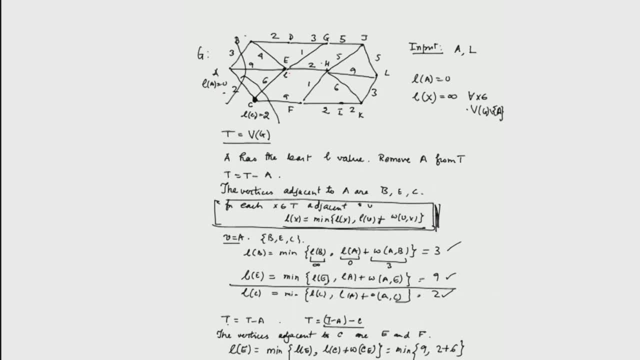 that e is now labeled as. level of e is equal to 8 and level of f is equal to 11 and level of b is equal to 0. So e remains at 3 and we have cut out c. Now we go to the next iteration, When we 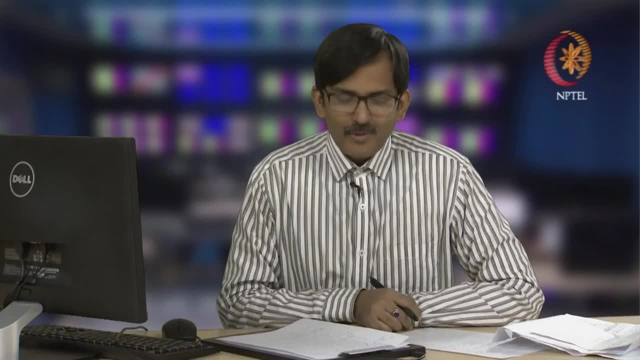 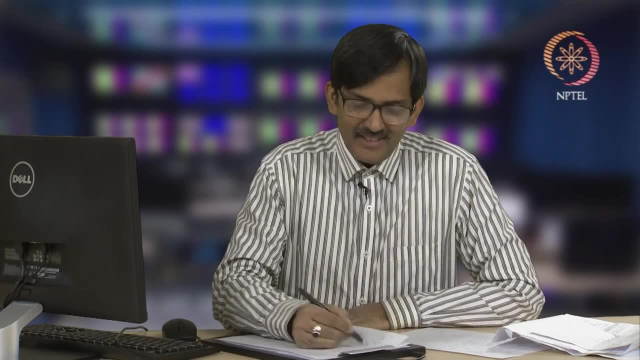 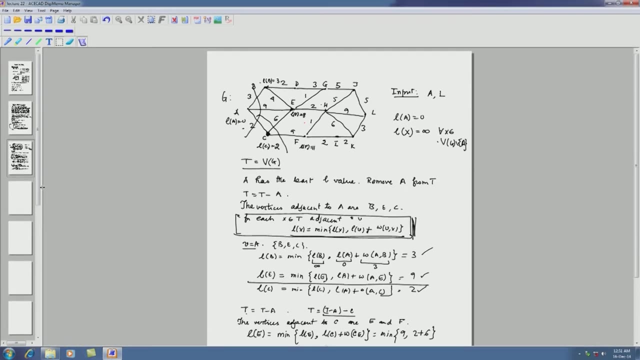 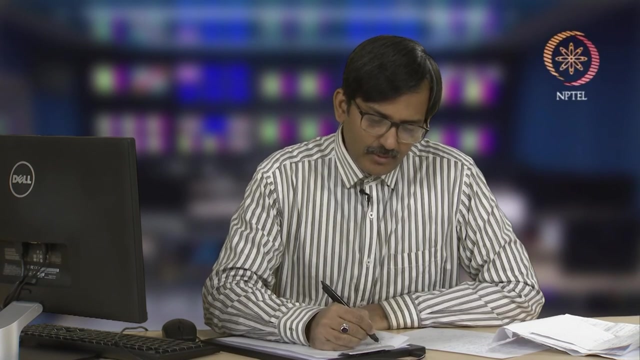 go to the next iteration. our vertices which we have to consider are b, e, f and rest of the vertices are infinity. Among them, we see, the b is the smallest. So we have cut out b and we have to start with b, which is 3.. So we are essentially cutting out b and then 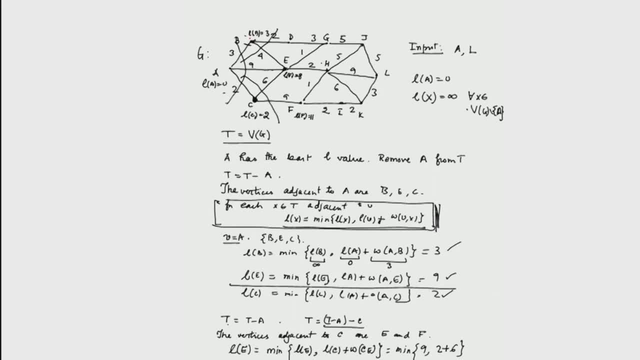 we are recomputing the levels, So b is adjacent to d, d is already infinity. So therefore this value, L d, is going to be 5 and when we come to the next iteration, we have to start with d. d is going to be 5, and when we come to L e, we will see that it is even shorter. 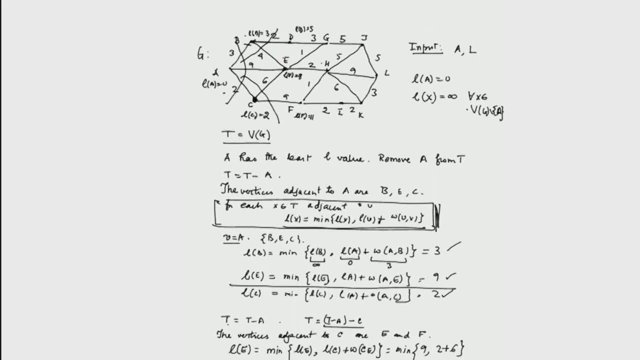 than before and because if we go from a to b, that is 3 and b to e, that is 7.. So I have to compare between 7 and 8.. So this value of L is going to change to 7.. So this: 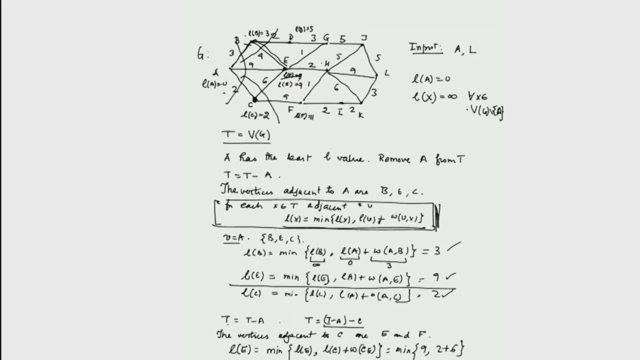 value of L is going to change to 7.. So I have got L e equal to 7 and L d equal to 5, and these are these are the vertices which are adjacent to b. So after we cut off b, then again we have to look at the graph. So I have got a- b. 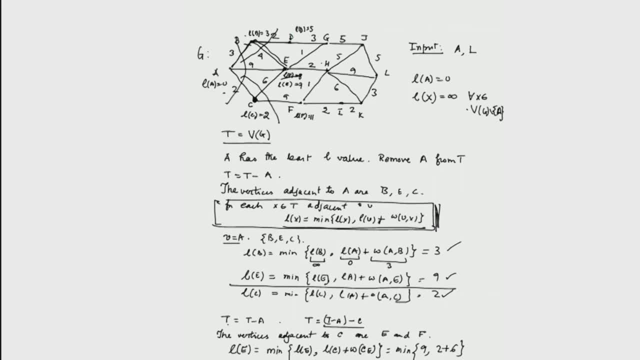 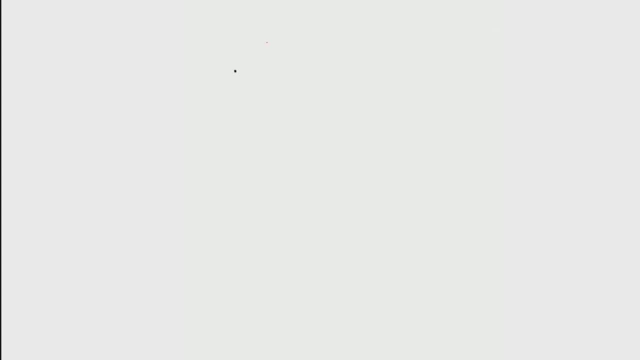 d, else a, c, f and a. So when this is a, this is a, a, b, d. there is a path of this: A, A, b, d, this is c, A, b, d. So when this is a, this is b, then again we have. 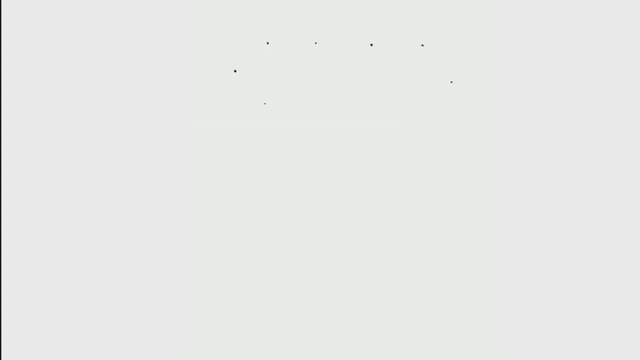 to look at the graph. So I have got a, b, d and b. So I have got c, b, d and a. So now we are actually: This is a, b, then we have d over here. 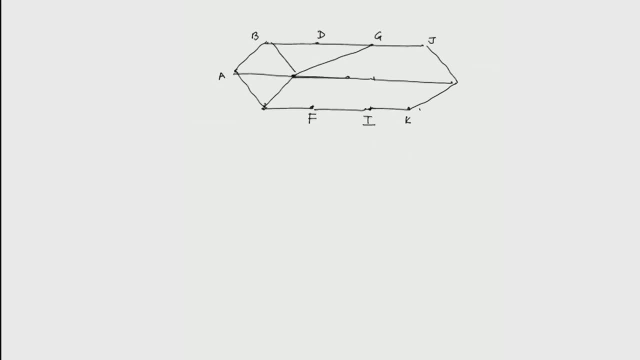 then we have g over here, j over here, l over here and c, f, we have e, and then we have h. h is connected to j, h is connected to k and f, both. and now the weights: we see that this is 3,, 2,, 4, and. 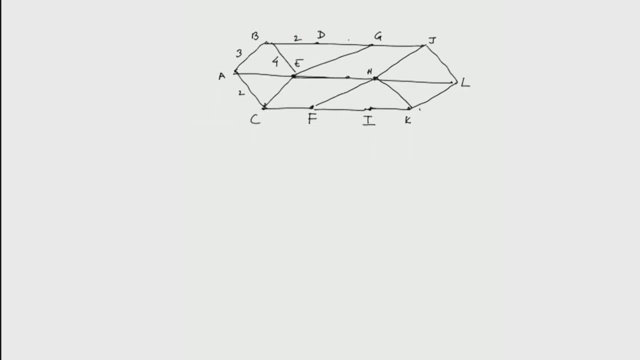 1.. This is 1,, 2,, 3,, 5,, and this is 1, and this is 5,. this is 5,, 3,, 9,, 6,, 2,, 2, here this: 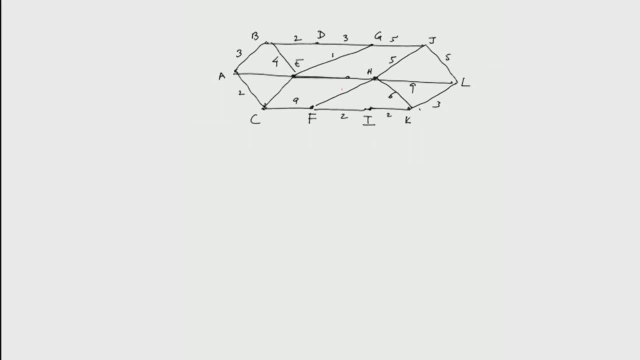 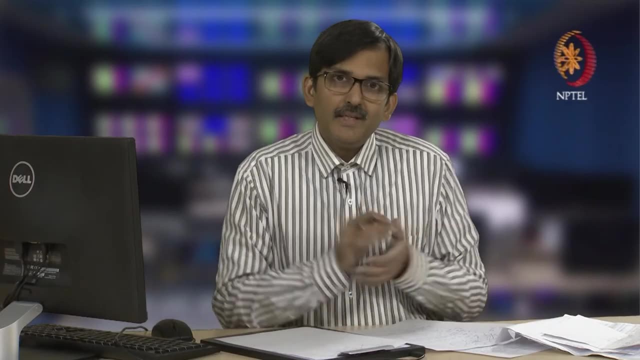 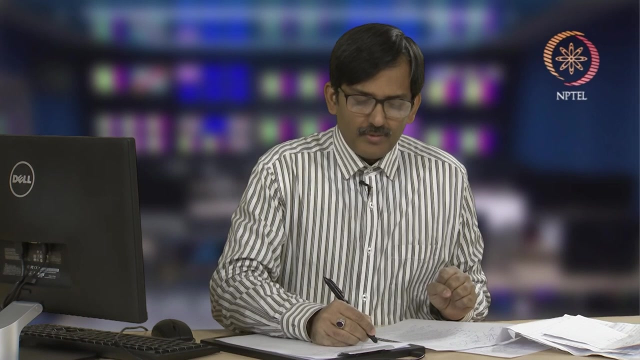 is 9, and this is 1.. Now what we see over here and this in between is 2,. now what we see over here that we have taken care of 3.. We have taken care of 3 vertices. l a is of course, 0 and we have, fine that, found that. 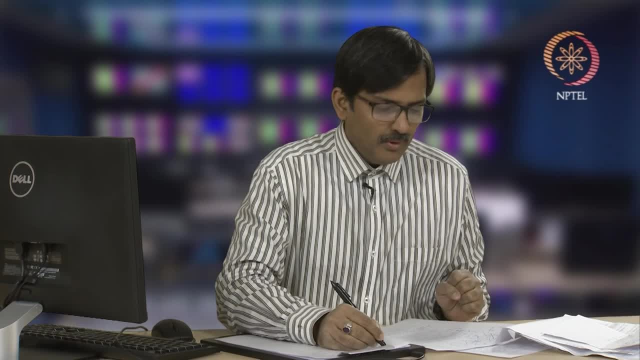 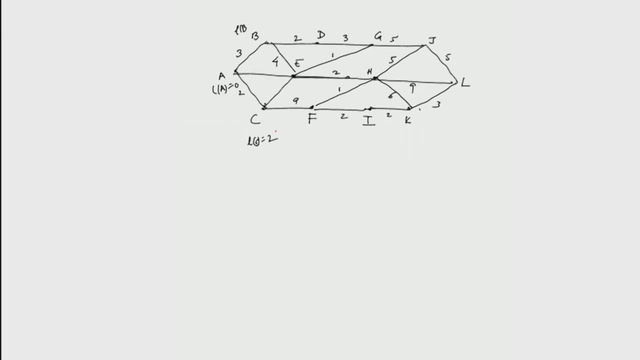 l b equal to 3, l c equal to 2.. These are not surprising, but because of our algorithm, we have come to understand that l e has a smallest value: 7. L d is equal to 5, L f is equal to 11.. Now if we look at this one, then we will see that 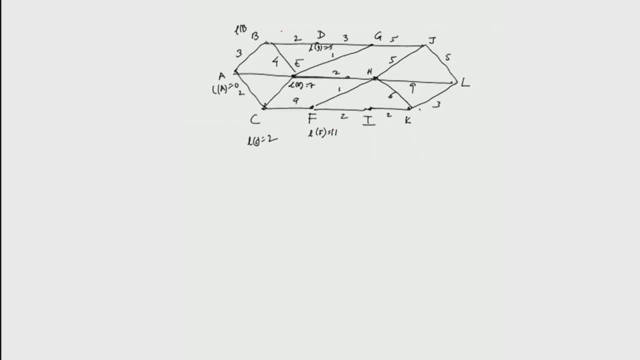 if we look at this one, then we will see that now I do not have to consider b, c, b a c. So now I will consider the values of d, e and f. So L d is 5, L e is 5, L c is 5, L d is. 5, L d is 5, L e is 5, L c is 5, L d is 5, L e is 5, L c is 5, L d is 5, L e is 5, L. 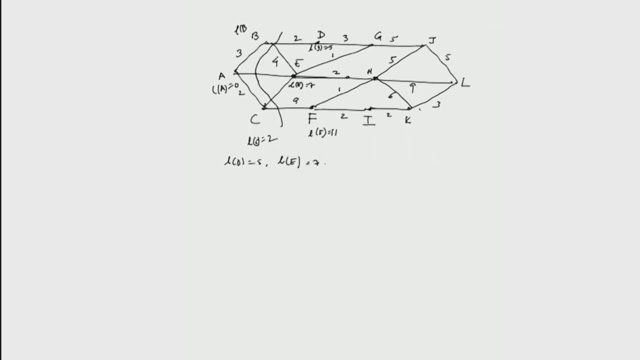 d is 7, and L f is 11.. Now, among this, of course, I will choose L d, So I will take out l d, So this also will go away. and then I have to find out the vertices adjacent to. 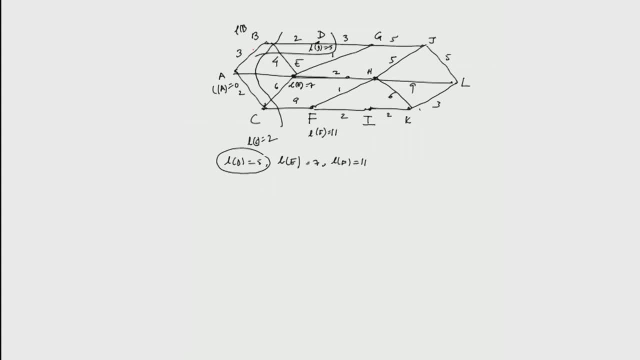 l, d, sorry, adjacent to d, and calculate its l value. The only vertex which is adjacent to d is g, and its l value is going to be 5 plus 3, that is, l g will be 8.. So this is going to be 5, and then? so I will go to the next step. Now I will have, I have to consider- 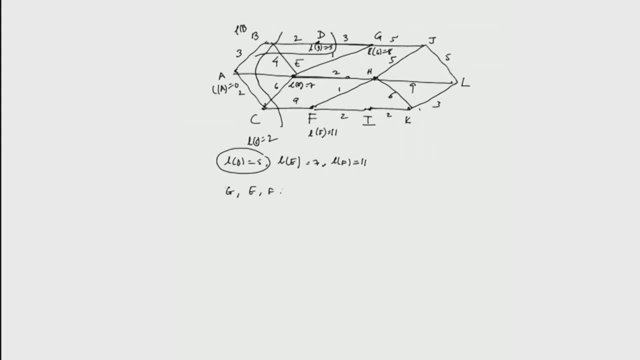 g, e and f. and when I consider g, e and f, then I am going to get e as the vertex between smallest level. So this is the vertex with smallest level. So I have to cut, yeah, So I have to cut out e and then consider the vertices which. 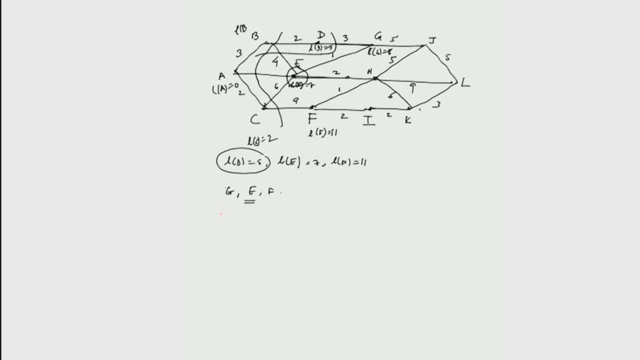 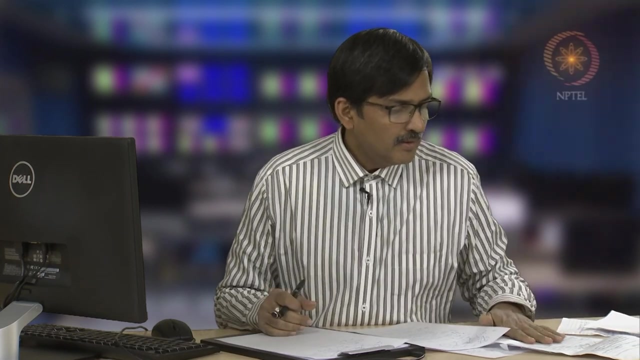 are adjacent to e. The vertices adjacent to e are h and g, both in case of h, e is 7, so it is 8, and this is 7 plus 8 is 9, so l h equal to 9.. So in this way we have to proceed, and if I keep on proceeding in this way, eventually, 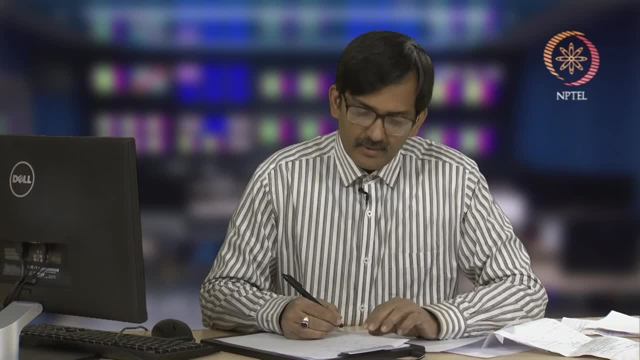 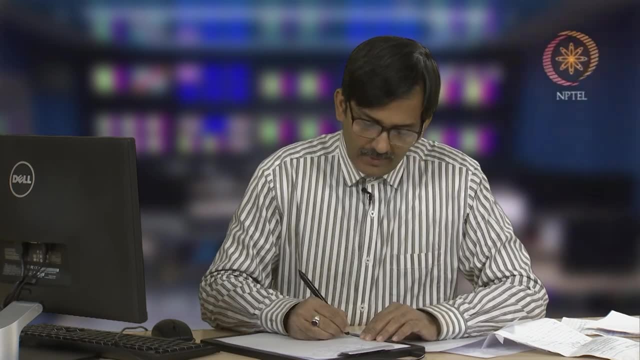 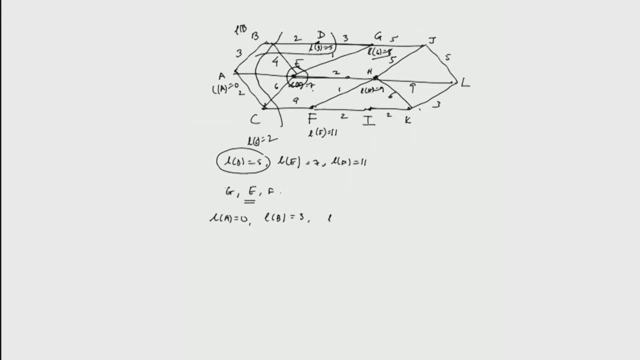 I will get the l values of the other vertices. We have given l values of several, but let me list down. I will get l a equal to 0, l b equal to 3, l c equal to 2, l d equal to. 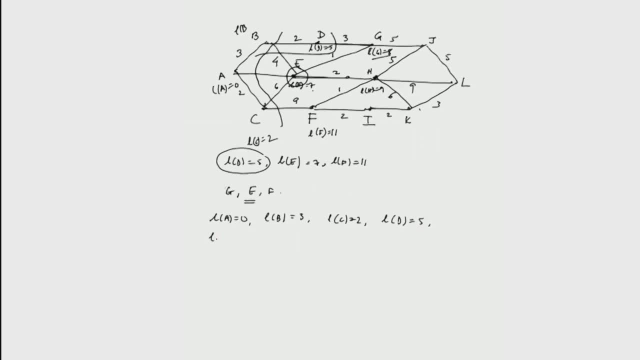 5, l e equal to 7, l g equal to 3, l h equal to 3, l h equal to 4, l h equal to 5, l h equal to 6, l f equal to it will come to 10, because we will find when we calculate from: 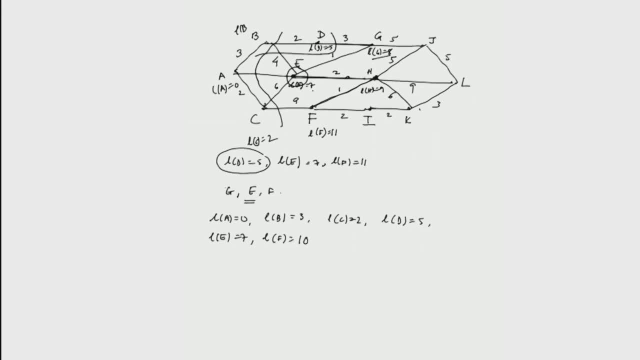 h, we will find that this is 1 and h is 9,. 9 plus 1 is 10, so l f will at one stage come to 10 and l g. l g will be 8,, l h will be 9,, l g will be 8,, l h will be 9,. l g will. 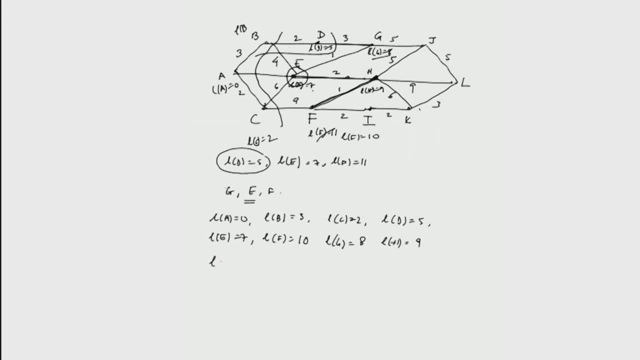 be 10, l? i? it will come to 12, l? k l? j? l? j will be 11, l? k will be 14 and eventually l? l will be 10.. will be 17, and what is the root for 17? we will have to go to b, then from b we will come. 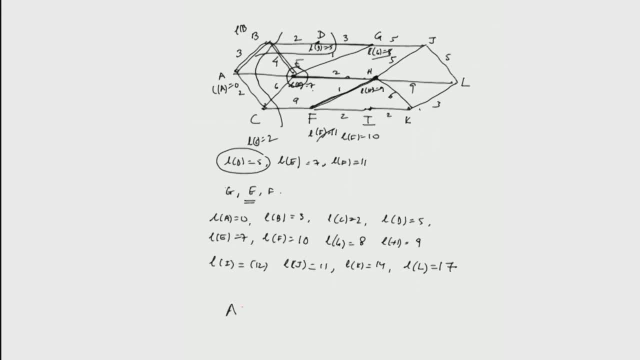 back to e, So a to b, b to e and then e to. we will go to h, like this: from h we will have to come back to f, So f value is 10, and then from f I will have to go to i, i to k and 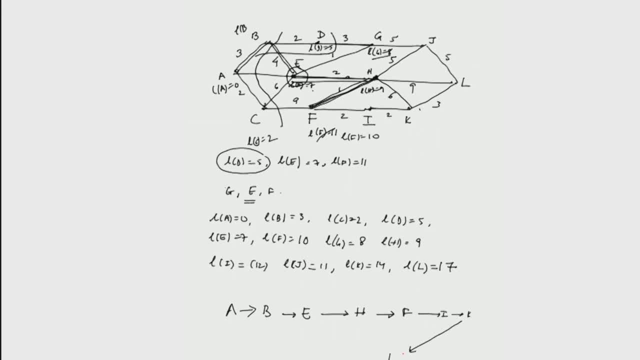 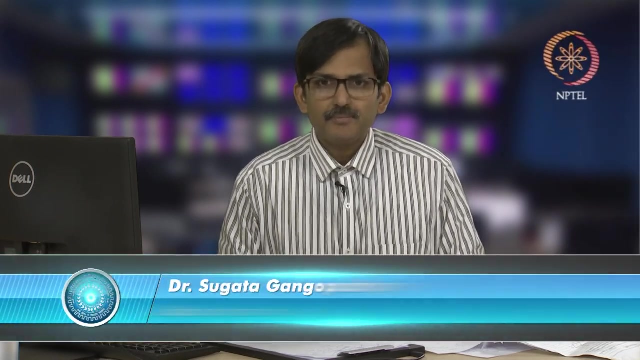 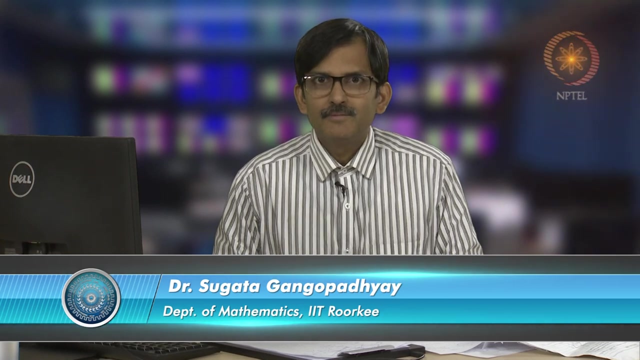 eventually k to l, So we see that l k is 14.. So l capital L is going to be 17, and that is the shortest path. We have to keep on doing, going through the iterations, and we will continue, We will get this. So this is Dijkstra's shortest path algorithm in action and this 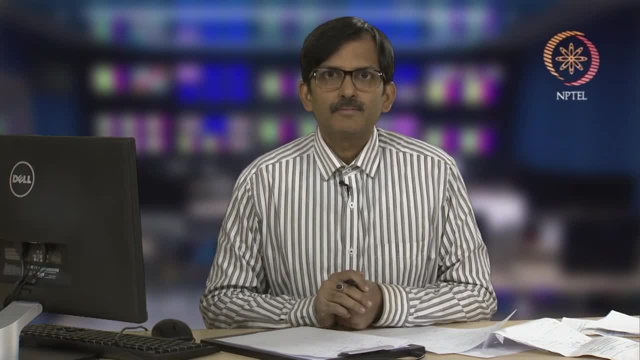 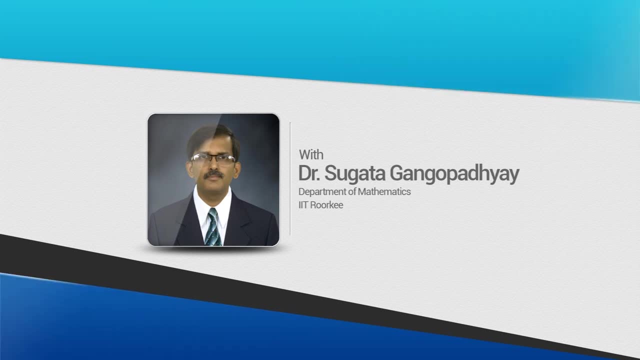 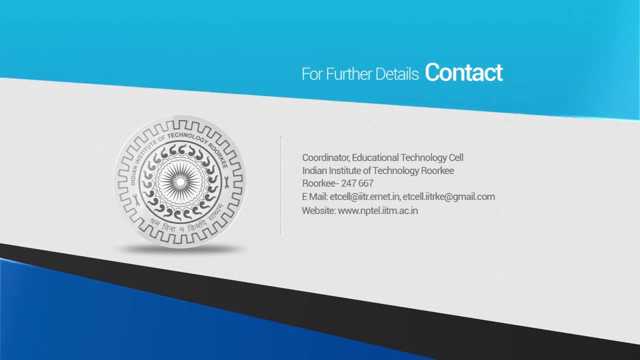 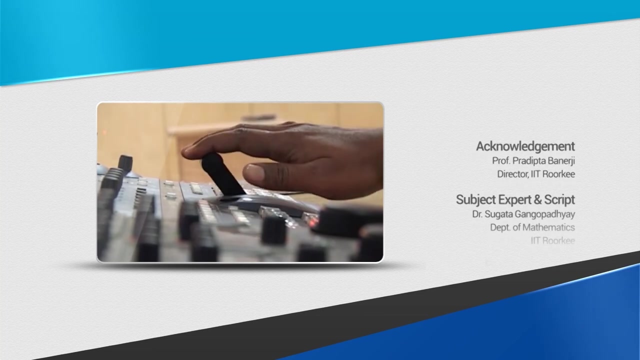 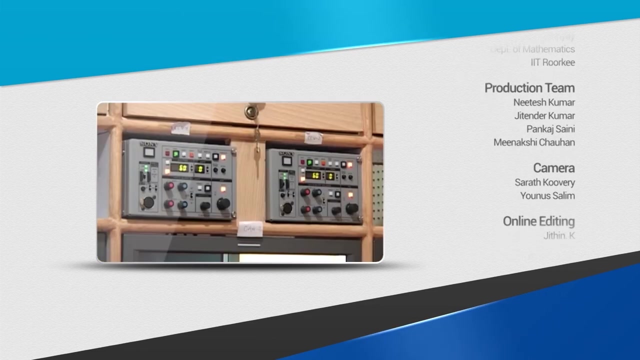 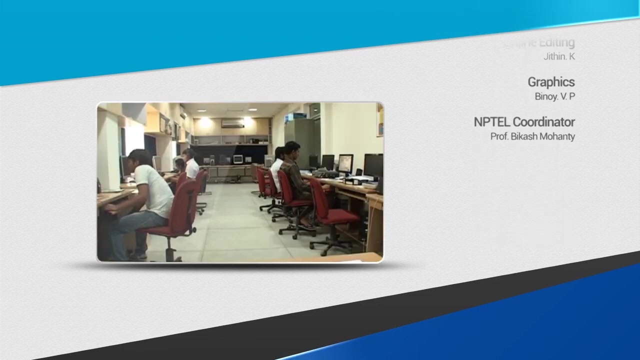 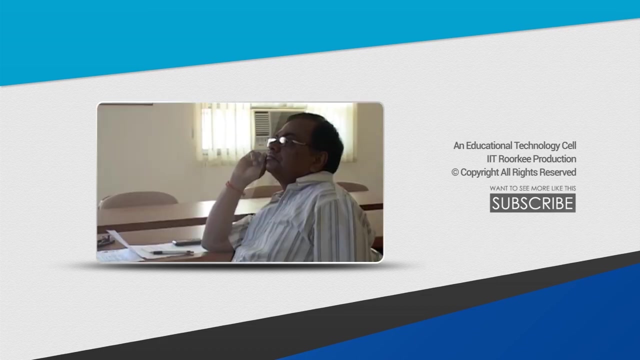 is the end of today's talk. Thank you, Thank you. 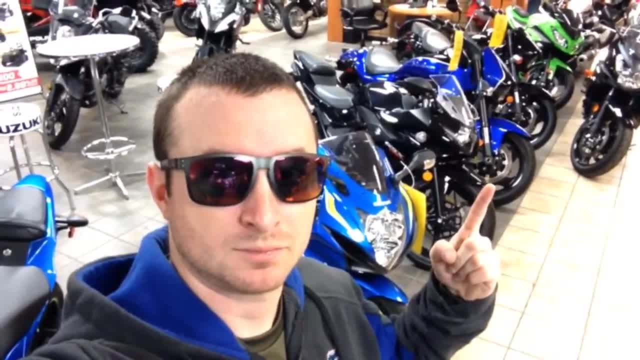 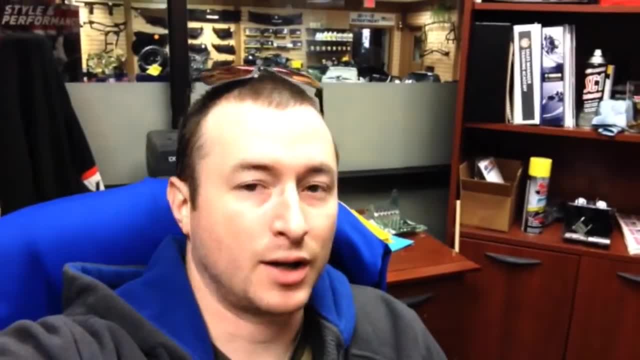 What kind of gas mileage do motorcycles get? What's up, guys? it's Alex. So one of you guys just recently asked me what kind of gas mileage to expect, or what kind of gas mileage you get out of a motorcycle, and the question was actually more. in relation to single cylinder versus multi-cylinder. that video I did, but I just figured I'd do a quick video to answer that and kind of cover all the bases on that. Simple answer is: gas mileage varies a lot across the board on motorcycles and it really comes down to a few. different factors and these are just very general rules. there are exceptions to them, but on any kind of bike- street bikes, what we're really covering here, on any kind of street bike, the more cylinders you have, the worse your gas mileage is going to get, kind of like on most cars. Exception to that. kind of being. also weight plays a factor. so but as a general rule you know a single cylinder bike is going to get better gas mileage than a two-cylinder bike. those are going to get better gas mileage on a three-cylinder, four-cylinder. you start getting your six-cylinder bikes. your gas mileage goes down some as a general rule there. are exceptions, okay. Other things that play a big factor in that weight: lighter motorcycle is generally going to get better gas mileage than a heavy motorcycle Size of the motor. you know, usually a smaller motor is going to get better gas mileage on a motorcycle, except if you've got a. working your motor at a higher rpm range. So you know your, your big single cylinder motorcycles usually get really good gas mileage. your twin cylinder motorcycles usually get really good gas mileage. when you start getting into three cylinders, four cylinders, etc. your mileage goes down. I've had bikes, you know, like Ninja 250s and other small bikes like that, that get as much as you know, 70 plus miles to the gallon. that's definitely reachable. on different bikes- Some of your parallel twin and single cylinder bikes- you can get 70, 80 plus miles to the gallon. and then I've had bikes like you know: my ZX6.